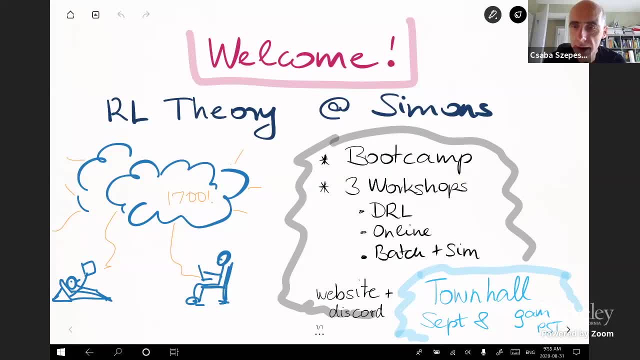 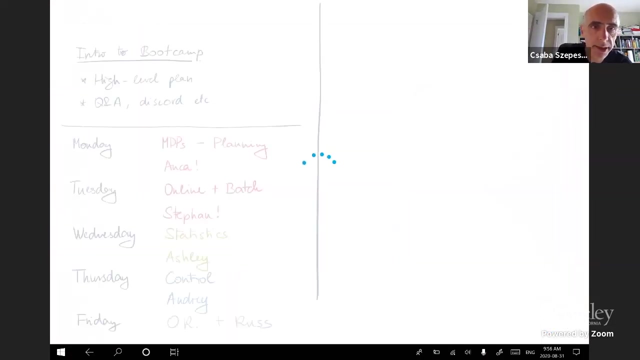 meeting on the 8th of September, That's next week, on Tuesday at 9 am to get really the program off the ground and do brainstorming about how to structure the program for ourselves. So with that let me go to the bootcamp introduction. 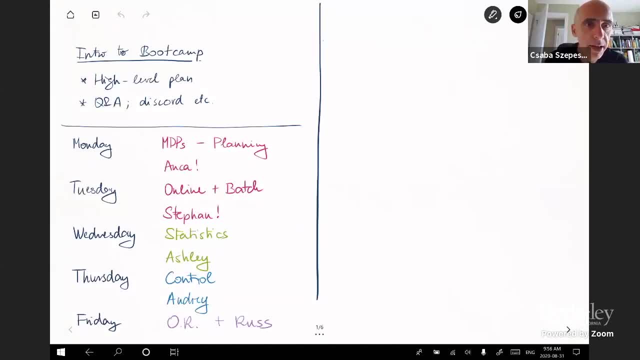 So this is the high level plan for the week. So on Monday you're going to hear from Mandy and me about the basics of MVPs and planning, And in the afternoon we're going to hear from Anca. So every day is going to be tutorials and then a bonus talk a little bit. 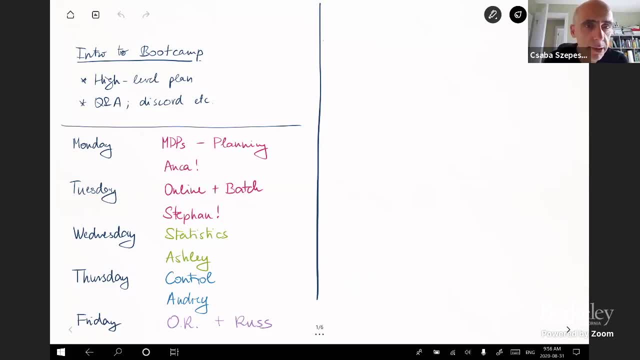 later in the afternoon. Everything's recorded. It's going to be available on YouTube, So we have to stretch across the globe by the time zones. It's going to be difficult, but I hope that we can include everyone. I see that someone has a question. Yes, 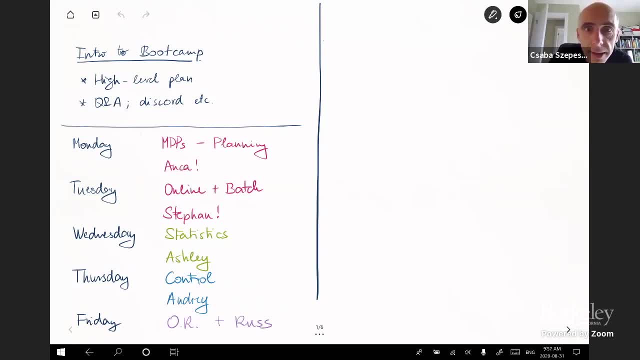 How do I see what the question was? That is feedback and two voices, one on top of the other. Not for me, Trevor. It's quite clear. Okay, All right, Okay, good, All right. So that's Monday, And on Tuesday: 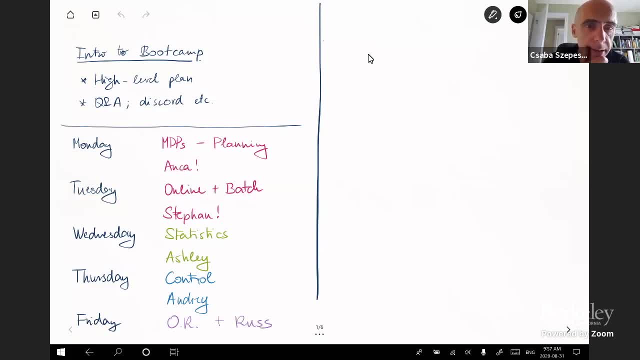 we're going to continue with online reinforcement learning and batch reinforcement learning. Stefan's going to give a talk in the afternoon On Wednesday. we will hear about reinforcement learning from statistics perspective, And Ashley is going to give the talk in the afternoon On Thursday. the control perspective And Andrea is going to give a talk on Friday: operations, research and RAS. 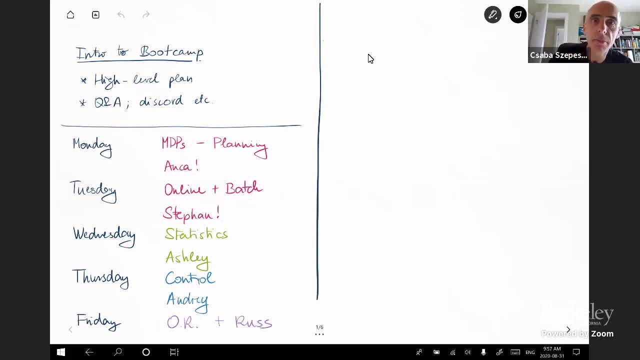 uh is going to give a talk. uh, so that's the plan. um, we want to uh keep this as much as possible interactive uh, so please, at any time, if you have questions, uh ask here. uh, either in the chat- i guess you can raise your hand or something like that. um, and uh, also, i asked uh the organizers to 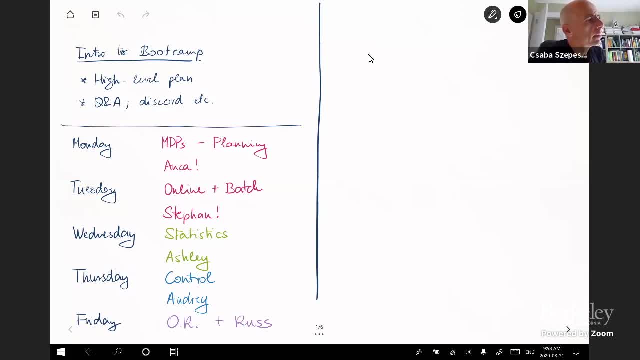 monitor the discord server, uh, so that if you have questions you can ask those. uh ask, uh ask the questions there and then, uh, someone probably going to raise their hand here and ask me the questions. so with that, i'd like to start with the first part of the bootcamp, which is mbps and planning. 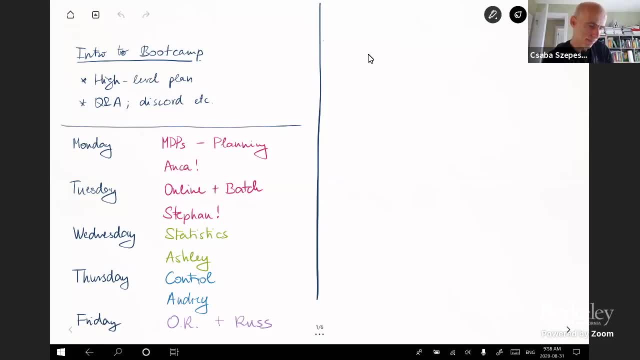 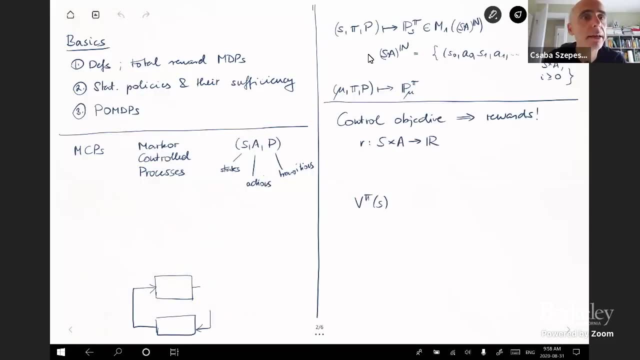 so so let's get started. all right, let's get started. so, um, the structure of uh. so i'm going to talk, uh about really basic stuff for about 30 minutes, uh, just introducing mostly definitions. uh, i was talking about definitions and and some some really basic results. 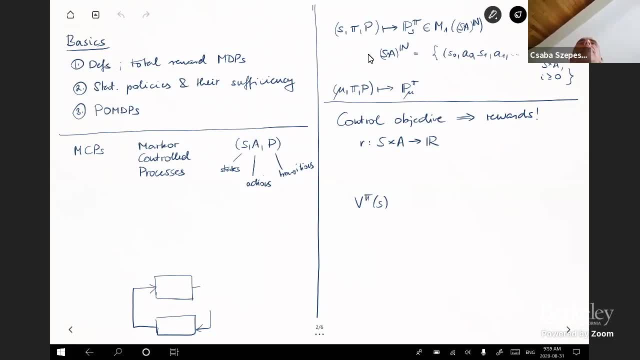 and then, uh, mangy is going to come in, uh, for 30 minutes, then we're going to take a break, and then mangy comes back after the break and then i will wrap up the morning. so at the very first, um, let me, let me see how i use this. 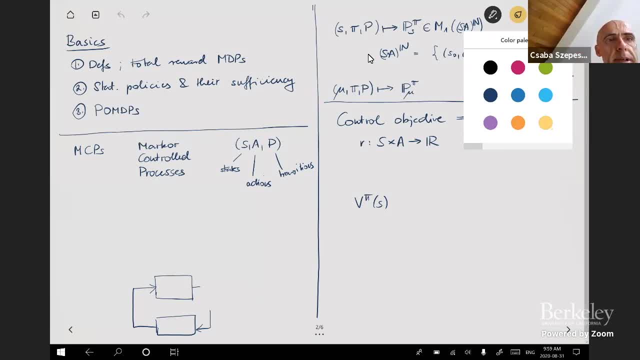 at the very beginning, i'd like to talk about uh definitions, uh. so i'm going to talk about mbps and total reward mbps, uh, and then talk a little bit about the sufficiency of stationary policies, what they are and and and in what way they are sufficient, uh. 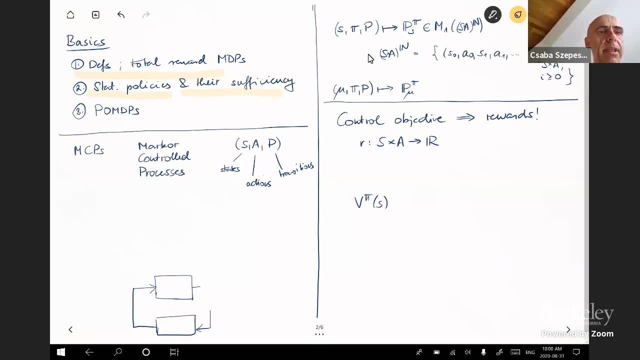 for mbps and then a little outlook at pump bps. so let's uh kick off, uh not even talking about mbps, but talking just about uh markov control processes. um, so markov control process is like an mdp, except that uh, we took away uh one piece of uh the mdp. 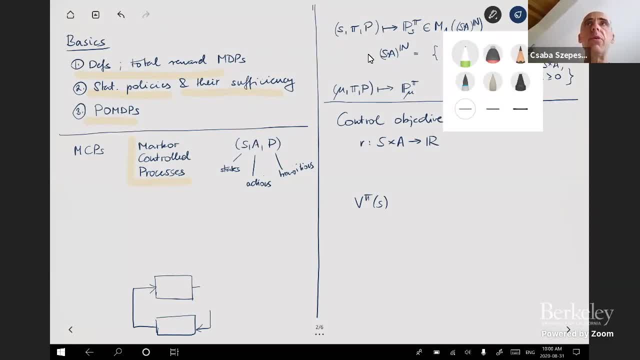 which is uh, which is the rewards. so what we're left with, uh are, are the states, um, and they're collected in a set. uh, i'm going to denote that set by capital s. so that's this set and, uh, we have a collection of actions, that those are collected in this set, a and 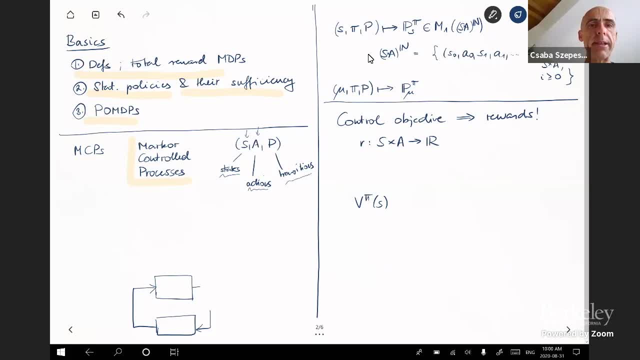 so the set of these set of actions, these are a collection of uh transitions. uh, these are collected into uh, this capital letter p. so what are these transitions? these are trans markov transitions. so this is a collection of um probability distributions, uh, one for each uh state. 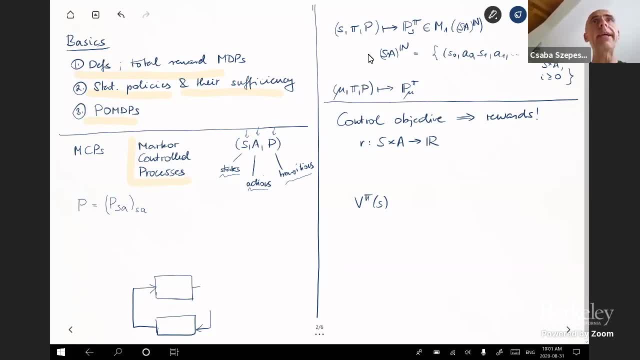 action pair. so lowercase s and lowercase a are going to denote individuals and next to it also states and actions. and to minimize clutter I'm very often just going to write S and A without a comma and without parenthesis and whatnot, So that means the same thing. 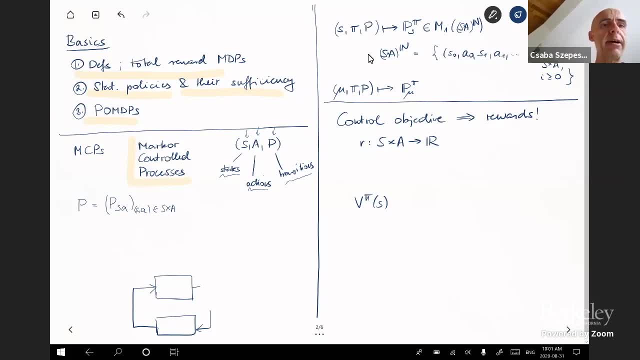 I just don't want to increase a lot of clutter, but everyone. so what happens here is that for each state action pair there is a distribution. So PSA is a distribution over next states. So if I need to talk about a distribution over some set, 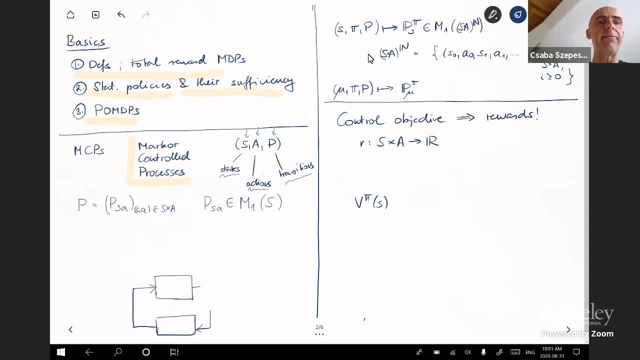 I'm going to use this notation of M1, of, and then in the argument, the set itself. So this is the collection of all distributions of this for every state action pair. we just have a distribution, And so the idea here is that 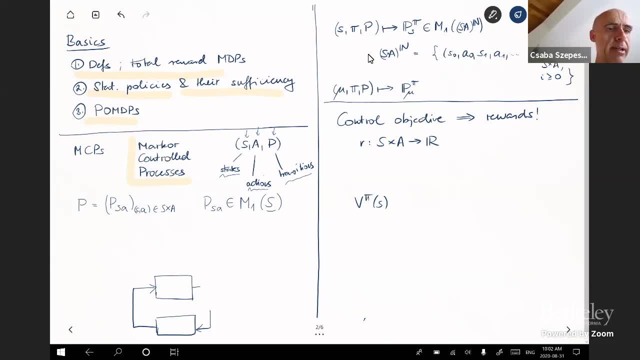 you start a process at some state, S is zero- and then somehow you determine some action- A zero, So that's coming from you, the controller, the agent or whatnot- And together this state and the action result into an next state. 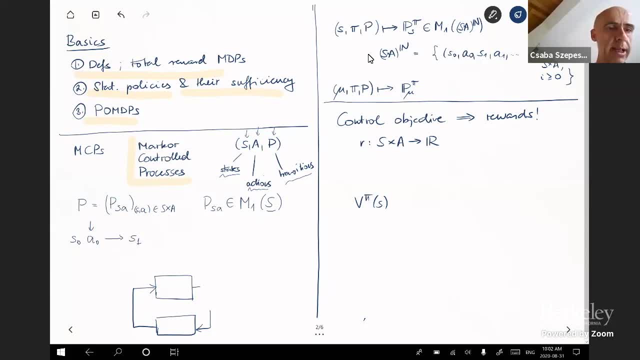 That's S1. And so this S1 is distributed according to this distribution: S naught and A naught, Okay. And then you come in, and then you choose another action, And when you're choosing this action, you could use basically the first state. 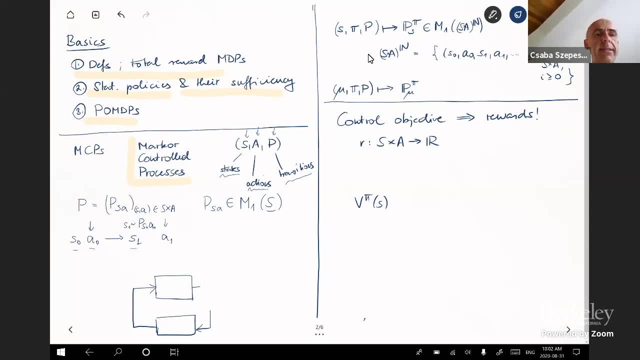 S naught and A naught and S1, the whole history. That's what you're gonna call the history, And this process continues this way. So in each and every arrow here, we're using this Markov transition kernel. Make this a little bit more orderly. 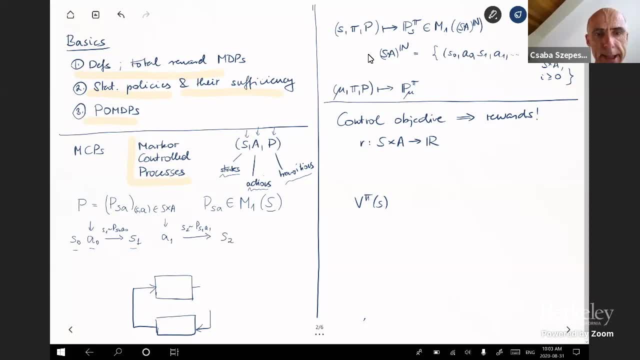 All right. so this results in this next state and then a new action is chosen, instance of force. So we can also illustrate this using a little diagram. So on the diagram. so time is discrete, So T goes from zero and then it's incremented. 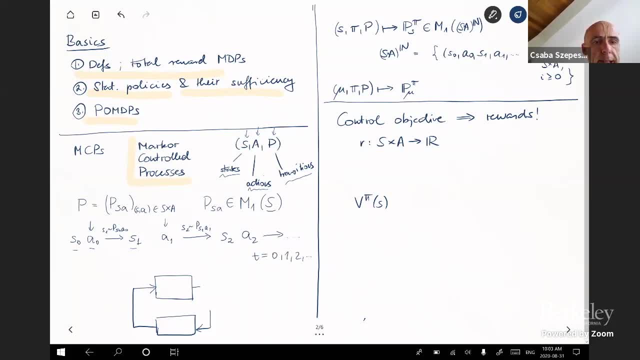 So by increments of one. So you started S T at time T and you have a little controller that can have some memory and it can also randomize- Today not randomization, but so this controller- we also call the maps- that it implements the policy. 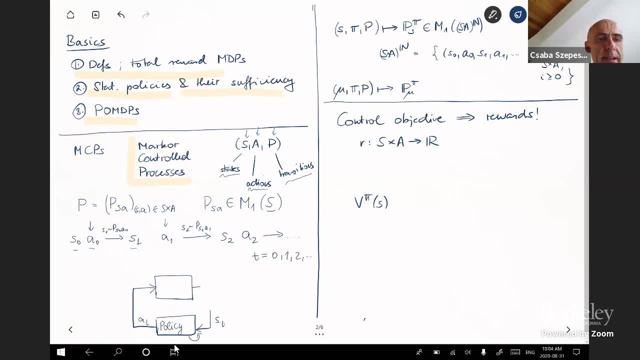 is going to compute eventually based on the information that we're able to get. So this is an action AT And this AT is fed into this system. So the and the system has its state and it's making transitions, these stochastic transitions. 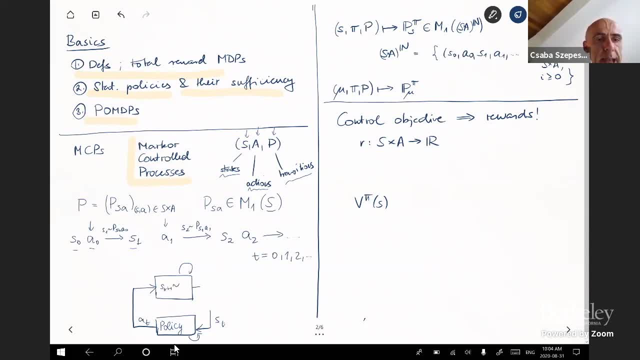 It makes a transition to the next state, which is S T plus one, And this is chosen from this PSTAT probability distribution, And so then this state comes out and it's fed back to to the controller and this way a loop is closed. 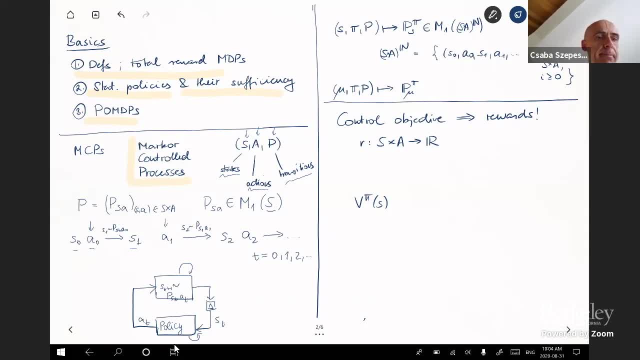 And these results in a sequence of state action pairs and infinitely long sequence of state action pairs. All right, You see that there are some questions. I don't know Why M one is just a function of the state space, Why M one is just a function of the state space. 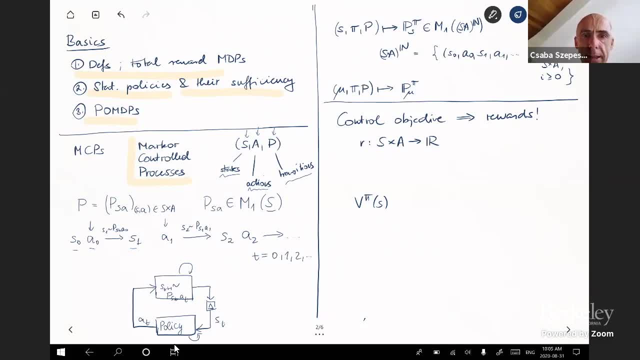 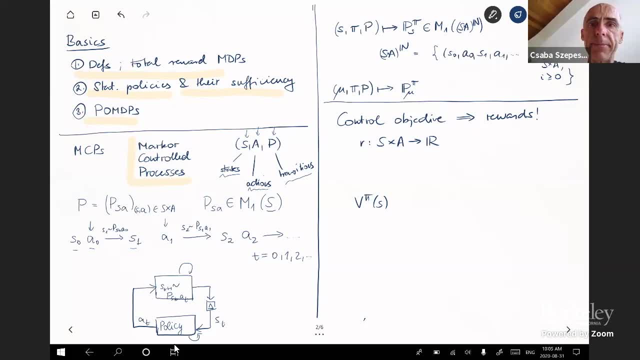 why M one is just a function of the state space. It's because these distributions are over states. I hope that now that I drew the diagram and we have this process view, it's clear that the action component is, you know, coming from the policy and the state, the next state. 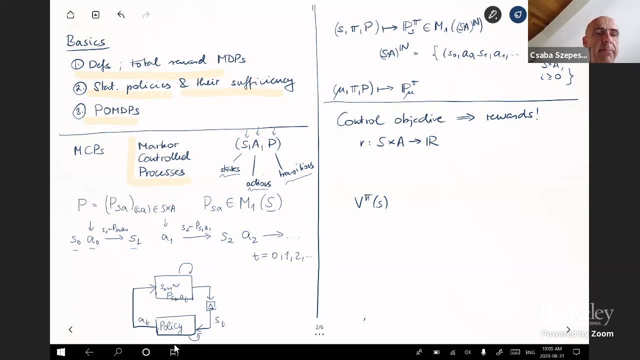 component is coming from the system that that is being controlled, And so this is called Markov control process, because the next state distribution only depends on the previous state and the action. So the control part is the action And the Markovity part is that you can discard. 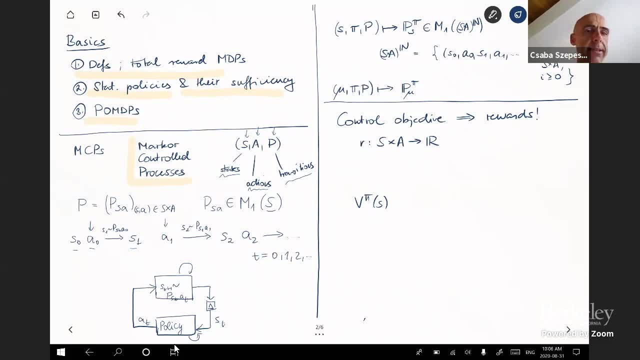 all previous states and the next state distribution is going to stay the same. Another question: Would you mind Could we go over the location of P again? So P of S of A, so for each action, pair S of A, that is, that is a distribution over the states. 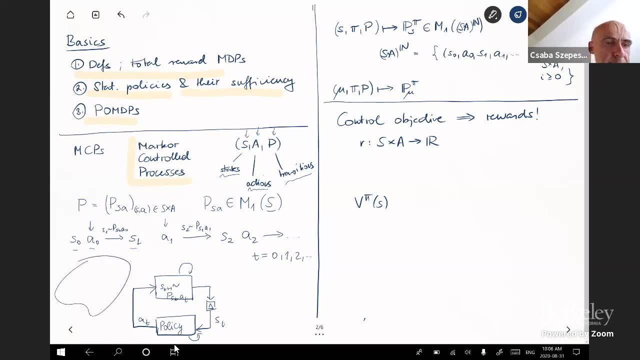 So you can also think about that. You have the state space here and then you are at some state and then you choose some action that comes from the different state, different space, And that induces a distribution over the state space. So you end up in this, this cloud. 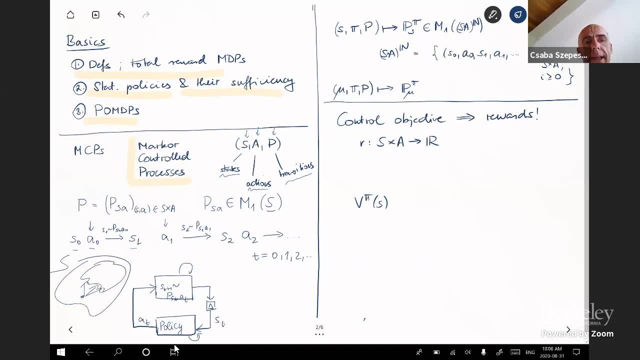 like, with some probability, you're reaching each and every state And then the process continues this way. I hope that this is clear. So in the Markov control process, so this M, we are given this S and A and P and we're just setting up things. 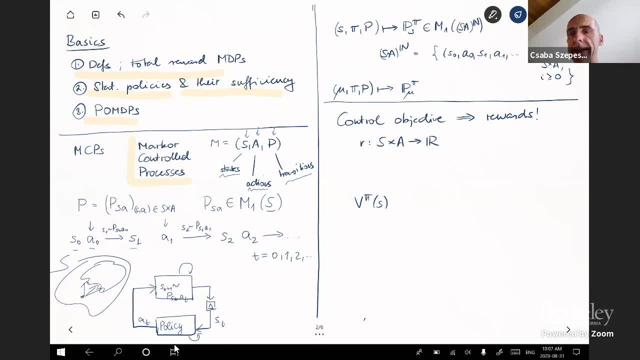 We are not talking about anything. you know we are not talking about anything. you know anything beyond that? Okay, So, given the state space and action space and these transition kernels- these are called Markov kernels as well, And if you have big spaces, then they have to have. 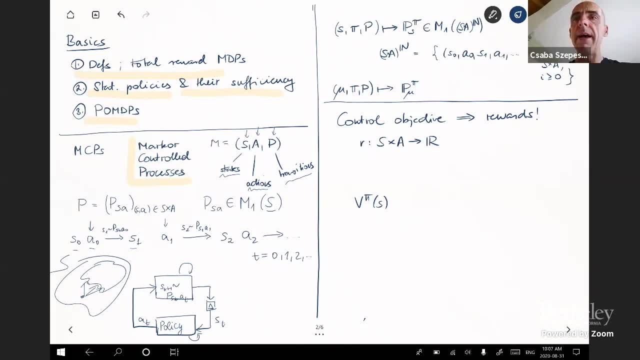 you know necessary measure with the properties, but that's, let's just disregard it for now for the sake of time. So if you've given this, then you can fix a given state and then you can choose a policy And then given the Markov transition kernel. 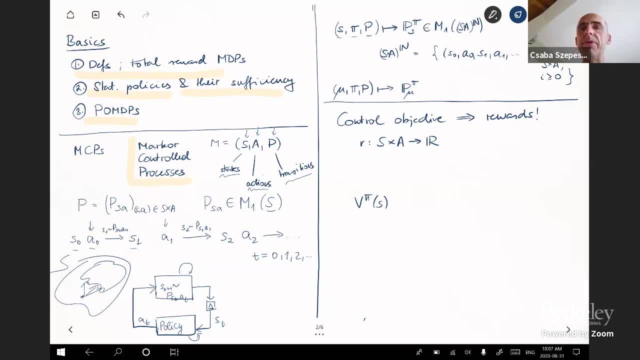 this results in a distribution over the space of all trajectories. So so this is the trajectory space. So these trajectories are these infinitely long sequences of alternating state action pairs, And I hope that it's clear how this distribution is constructed. The distribution on each and every component is: 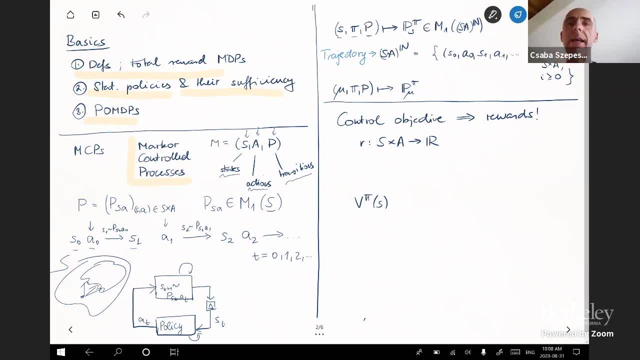 you know, like an S naught, that's a bit of distribution put at S and A naught is determined based on the policy It's distribution and S1 is determined based on- you know, like it's here- based on the transition kernel and so forth. 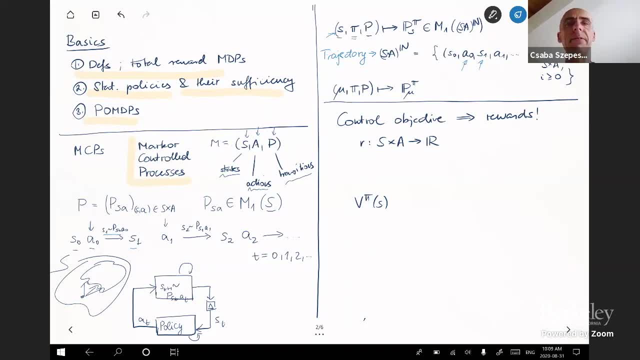 You take all of these probabilities if you're in a discrete setting, and then you multiply everything together and that gives you the probability of trajectory. And if you are in B0, in bigger spaces- then you can do this, extend this idea to these bigger spaces. 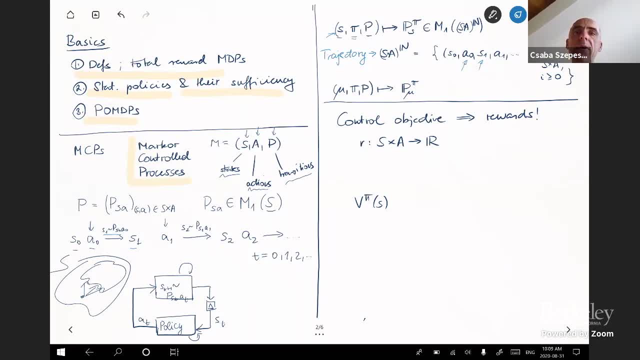 in an appropriate manner, And so here the important thing is that I'm going to use this notation of P, of S and Pi, which is a distribution over these infinitely long sequences of state action pairs, these trajectories. So these are distribution or trajectories. 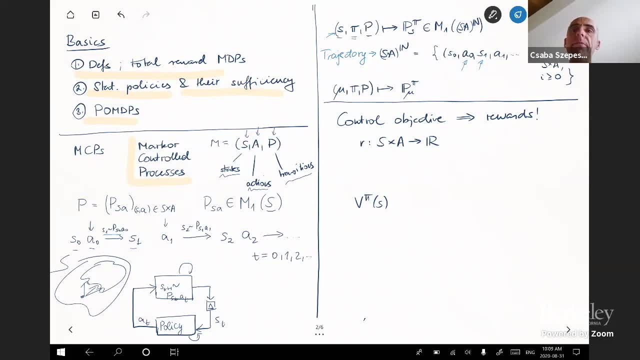 And if you have a probability distribution, distribution, and of course you can introduce an expectation operator and I'm going to use similar notation for that. So this is going to be the underlying expectation operator. And if we have an initial state distribution, mu- so here mu is a distribution over states. 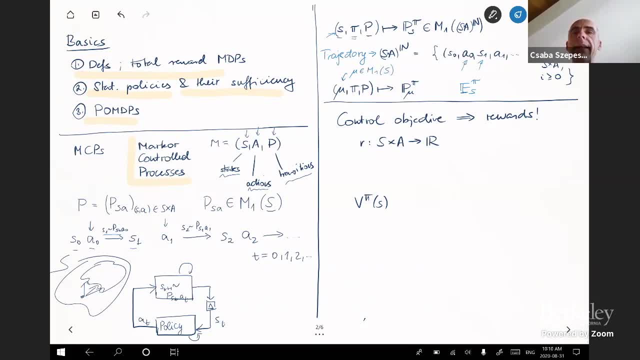 then a similar construct leads to distributions over trajectories And similarly we can introduce this expectation. operator p of u of pi. All right, I think I did answer pretty much all the questions. I would say I don't understand. Someone said yes or no. 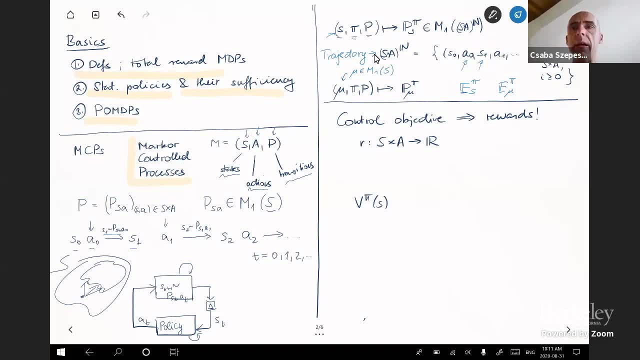 All right, Okay, So we have constructed this probability distribution, given an initial distribution or initial state policy Markov kernel over the space of trajectories. So what are we going to do about it? So we need a control objective. For the control objective, we're going to use rewards. So we pick a reward. 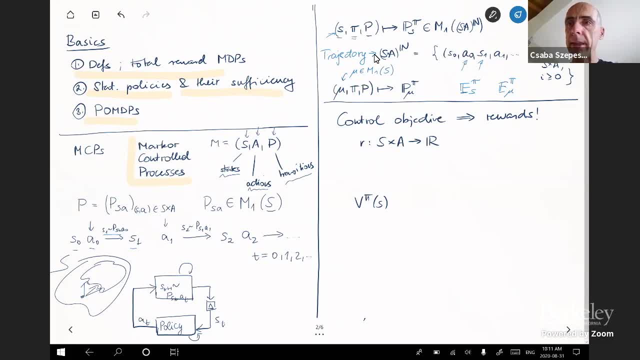 function R. So this is your reward. function R, Sorry, Okay. So it maps state action, pairs real numbers. So this is my notation for the numbers, And so if you have a trajectory, I'm also going to denote trajectories by just age. So if you have this directory, 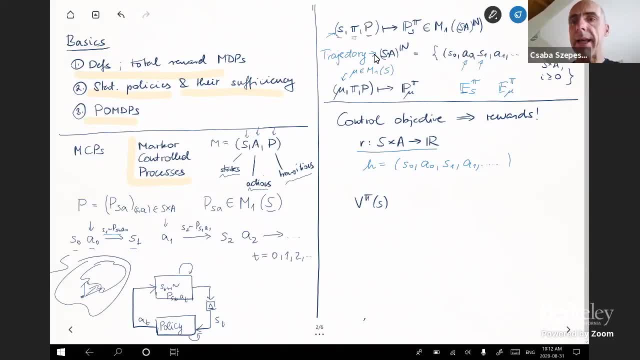 then you can assign a return to the trajectory, which is just the sum of rewards along the trajectory. It's an optional discounting, So these are called. this is also called the immediate reward function, because you receive these when you're making a transition. 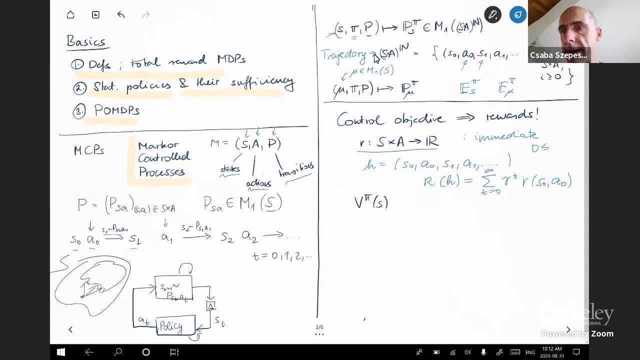 And here this gamma is this discount factor, And many times we choose it smaller than one, And if the rewards are bounded, then this would ensure that this function over the trajectories is well defined. So capital R is the return function And this sum is just called the return. Okay, So once we have the return we can define. 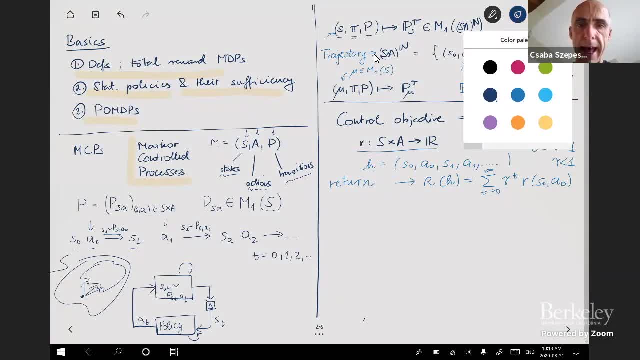 the value of a policy. So the value of a policy is, if you start a policy at a particular state of S is denoted by V of PI of S and it is defined as the expected value of the return. OK, That's all. 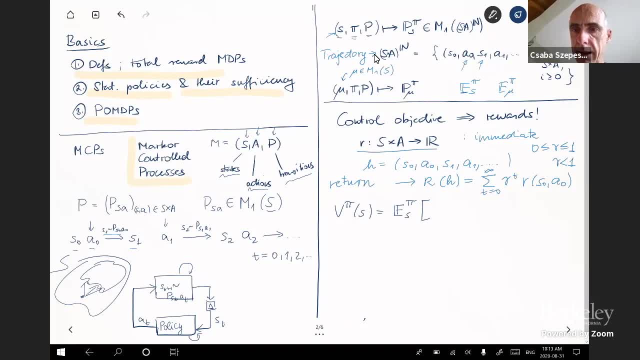 OK, So that's the end of the lecture. See you next time. Bye, okay. so so recall that. uh. so this p is uh the probability measure over the trajectories, and so this is this is basically uh. if you have, you know, uh, uncountable many trajectories, then 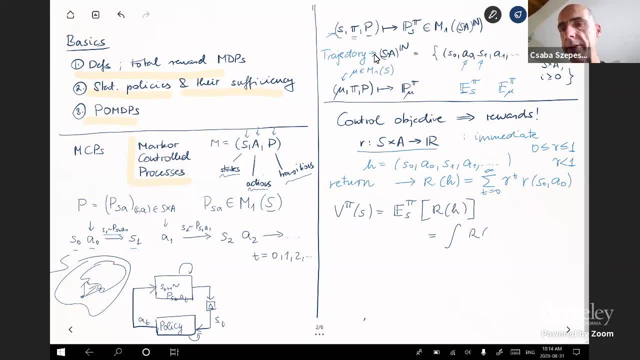 you would need to use an integral notation. so let's, let's go that way. uh, but uh. if you have finitely many uh state action pairs, then you can just uh enumerate all the uh trajectories- there is going to be countable many of them- and then this integral becomes just this sum. 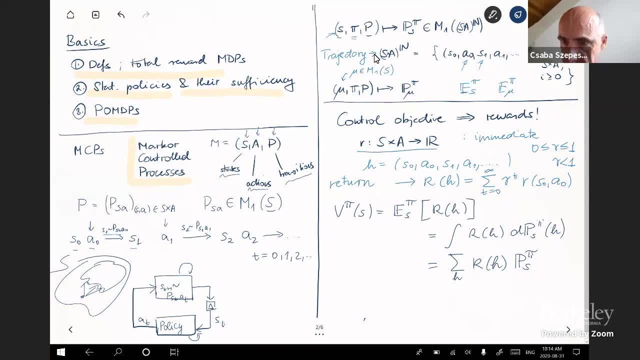 all right, there is some b that is annoying. uh, but i don't know about that. sorry about that. um, if i knew what is the source of that b, i would get it up, it's for sure. um, anyways, um, so, um, so this is the value function. uh, so i'm sorry, uh, so this is the value of the. 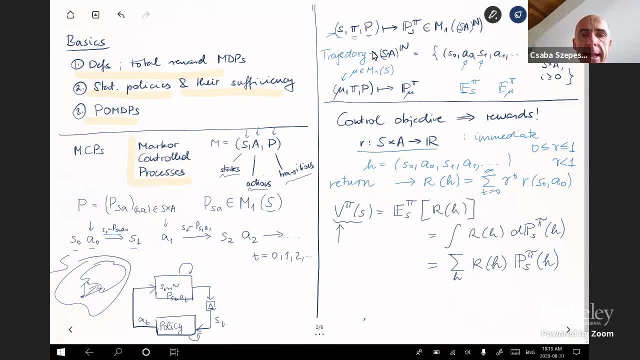 policy pi in state s and if you collect all these values, then v of pi uh can be viewed as a function that maps a state to an area of value. so this is going to be called the value function of a policy pi and there are many variations uh. so the variations uh would include uh, you know. 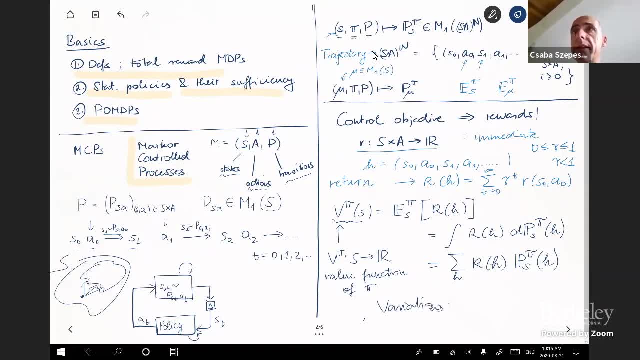 there is no discounting. there is discounting, okay, maybe, uh, the horizon is going to be finite. so, uh, maybe it is finite or maybe it is infinite. and sense of force, uh, sometimes, uh, you restrict the set of actions that are available at the given state and you have this admissible set of actions. 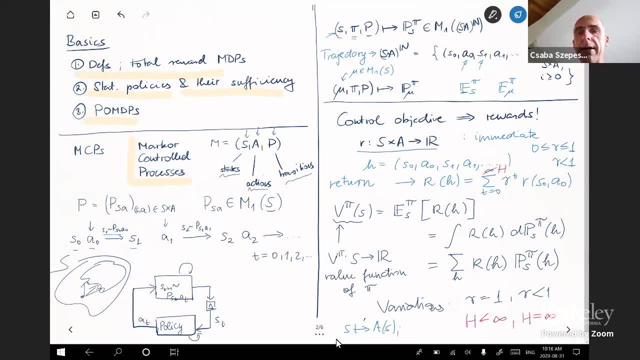 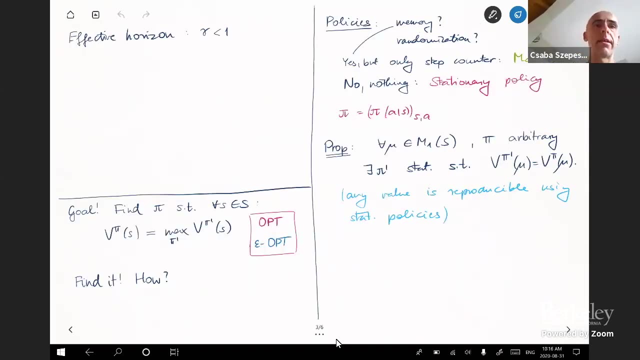 and sometimes you consider other criteria, like the average cost. i'm not going to talk about this. it would take too much time to to talk about this. um as well. all right, so, um, the control objective, um is shown here, um in the bottom, so let's let's focus on this. 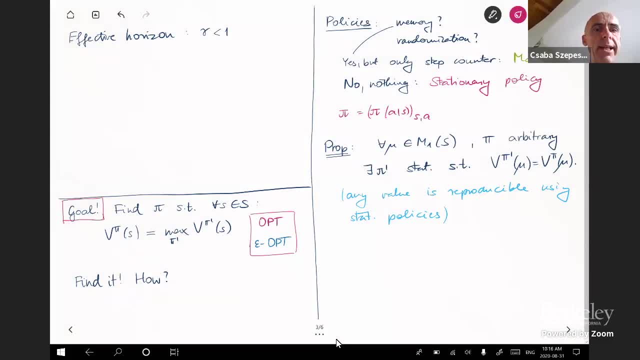 so the control objective is to find a policy pi, such that for every single state this policy maximizes, recognizes the values that can be achieved if you're free to choose a policy, even depending on pi. So this value, here this is defined as the optimal value function. 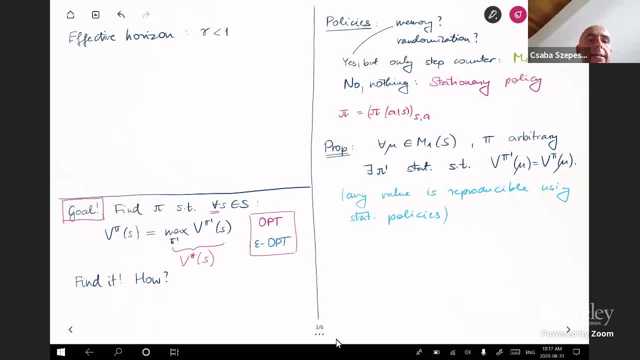 or the optimal value at state S to be precise, And if you collect again all of these values together, then you get V star, and V star is just this map that maps states to reals, And this is called the optimal value function. And solving NMVP means that you are able to find: 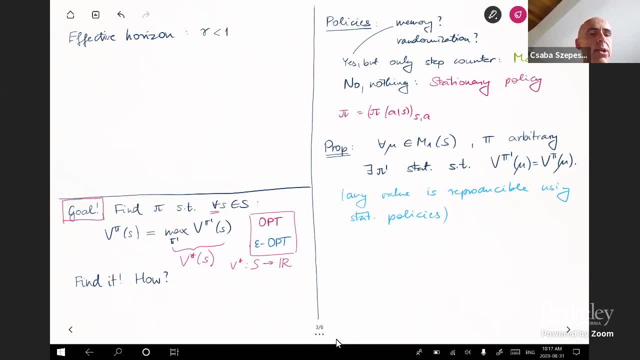 a policy pi, such that this policy achieves the best possible value at every single state. So in planning, you're asking the question of like: how can we do this? So planning asks the question: given an NMVP, what is a computational procedure that gives us an optimal policy? 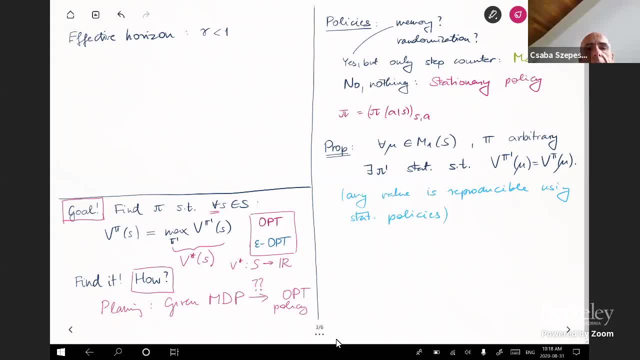 So how do we get a procedure? And so when we say that we are given an NMVP, I'm not too clear about what I mean about that. So in the next part Mengdi is going to talk about, the key is when we have a finite NMVP. 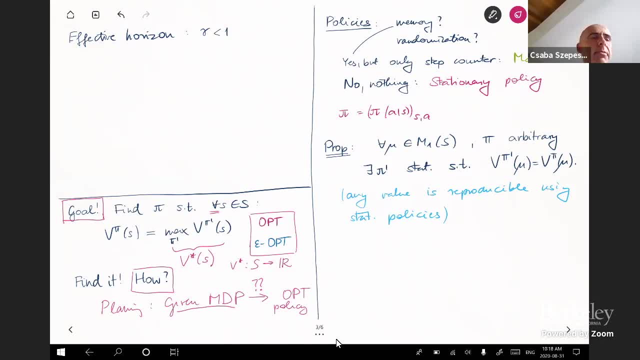 So, in this case, the number of states, the number of actions is finite and you can animate it. you know, like this state transition matrices, they just become a big table and you can animate everything. The value functions become vectors And you can, in this case, talk about that. you can find. 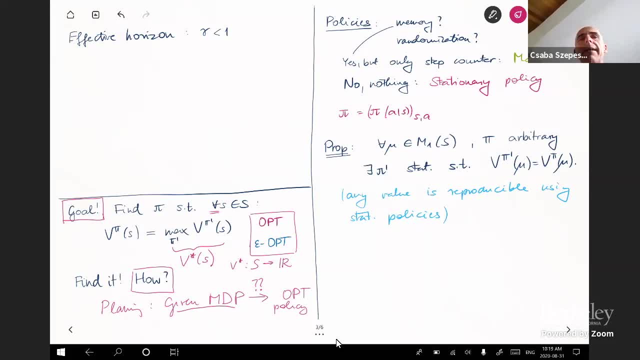 or not an optimal policy, and how long does it take to find such an optimal policy, given the information that is fed to you? So the information could come in this form that you're giving these big tables, and it's a good thought exercise just to think about how we would do this computation. 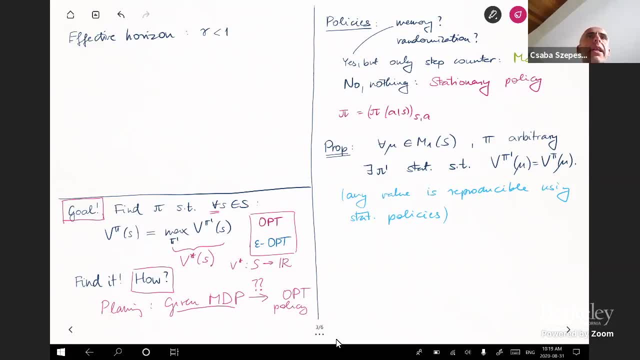 But of course that's not really practical. Many times we have much bigger number of states and also like action spaces, So that this enumeration is not practical. In the last part I'm going to talk about what we're going to do in those cases. 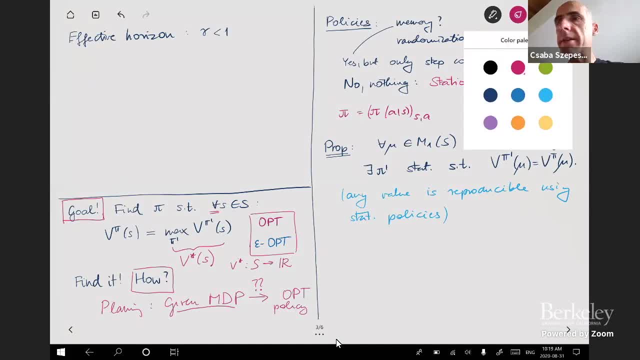 Before that, I just briefly wanted to mention one thing about effective horizons and discounting. If you have a discount factor and you're shooting for an epsilon- accurate evaluation of a policy, then what you can do is that you can cut this infinite sum. that was. 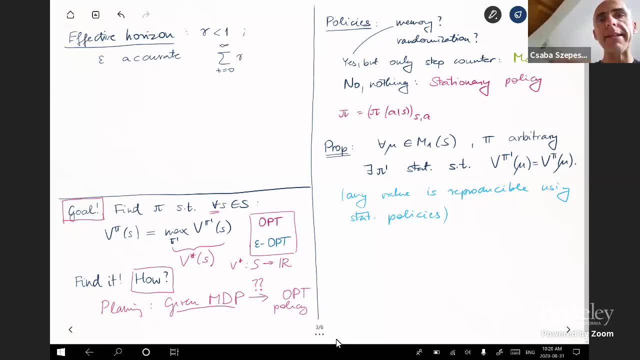 so in this case the horizon was infinite. So you can cut this infinite sum, You can apply the And at some finite horizon, this H gamma, and you can set the age karma to be like log one over EPS it on one minus the gamma, divided by one minus the comma. 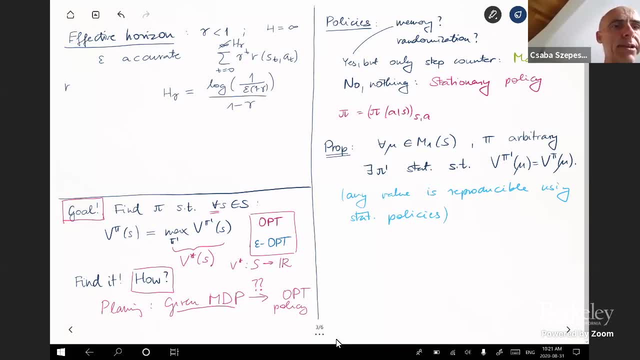 And so if the reward for that is not negative, then If the reward function- I'm going to assume this- takes values in the zero one inter log, then this ensures that you don't lose much by cutting the trajectory short. And so here this H gamma. 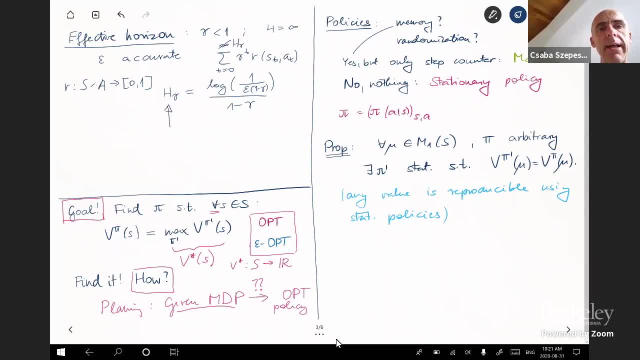 sometimes it just like one over, one minus the gamma, ignoring the log- is called the effective horizon. So this is just based on, you know, like taking the maximum values here, which are one, and like the maximum differences that you can get and summing the infinite series. 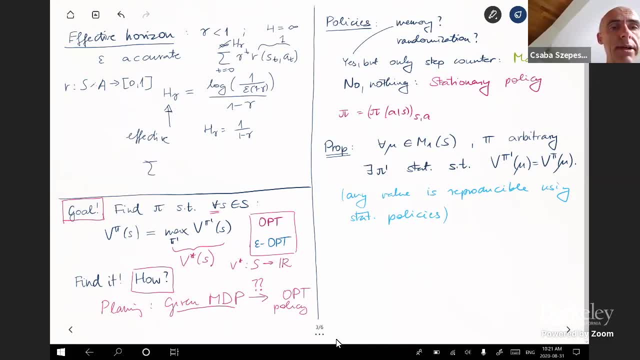 from H gamma plus one, sorry from. And so this is just going to be gamma to the power of H gamma plus one times one over one minus the gamma, and so if this is smaller than equal to epsilon, which is ensured by this choice, 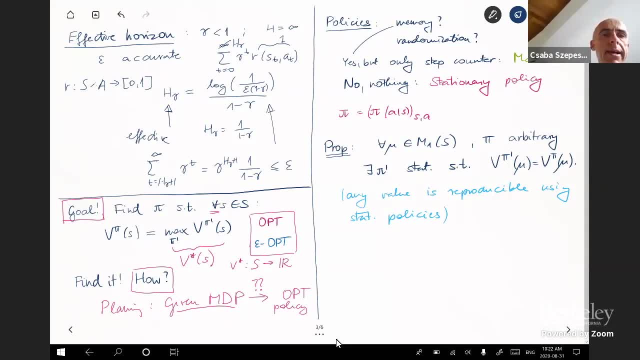 a little calculation shows that, then you can be sure that you're not missing much in terms of the rewards. And so if you're interested in absolutely accurate evaluation of your policies, then the lesson is that you don't actually have to consider infinitely long horizons. 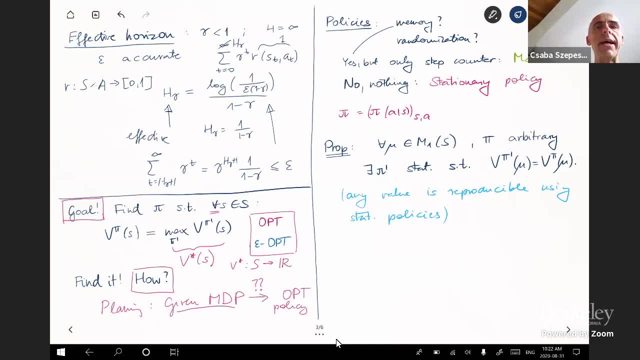 but you can cut the horizons short, And this is used a lot in a lot of different arguments. That's why I put this up first. So now the next topic is okay. so we set out to find an optimal policy, or maybe just an absolute. 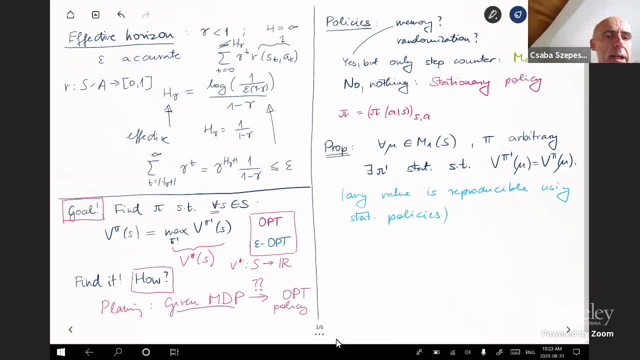 So I didn't say much about that. but the absolute optimality would be to find some policy pi such that V of pi is bigger than equal to V star minus epsilon. And let me write this one. So this is a vector notation. It means that for every state, 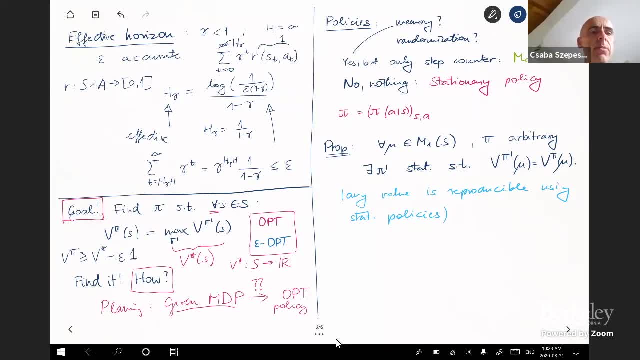 the value of the policy would be above the optimal value minus epsilon, So that would be the absolute optimal criteria. And so the question is: in what form should we search for policies like this? And, in a nutshell, the answer is that we should. 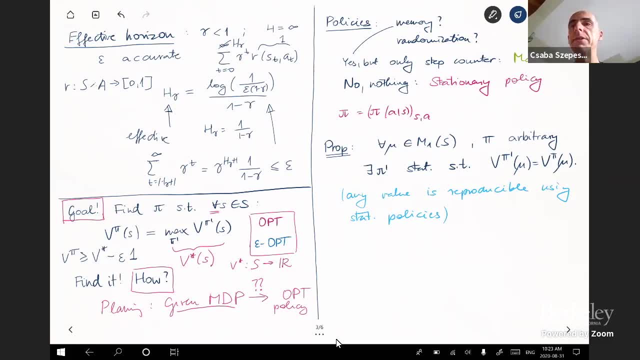 it is sufficient to just look at stationary policies. So what are these stationary policies? So a policy could have memory, could use past information, previous states and previous actions when it comes up as a distribution over the next states, if it uses randomization. 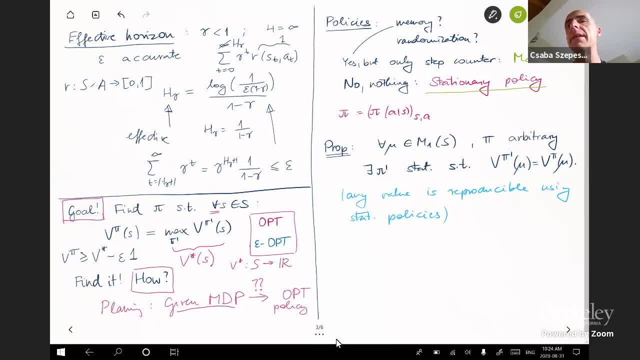 or it could be deterministic. So it may or may not use memory and may or may not use randomization. So let's first stick with randomizing policies. If the policy uses memory but only step counter, so it remembers like how many steps we are in the process, 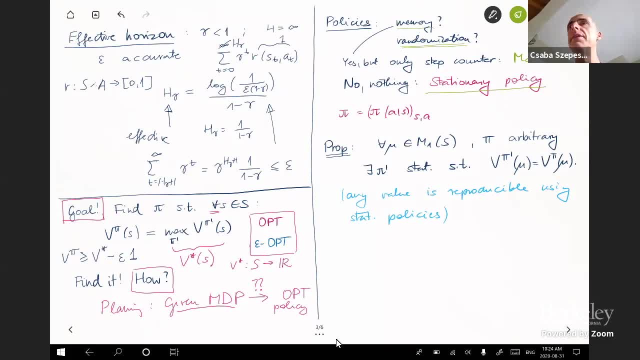 And, depending on that, it chooses a distribution that is based on this counter and the last state and the distribution is over the actions. So then we're talking about Markov policies And a policy which is a Markov policy which doesn't use the counter. 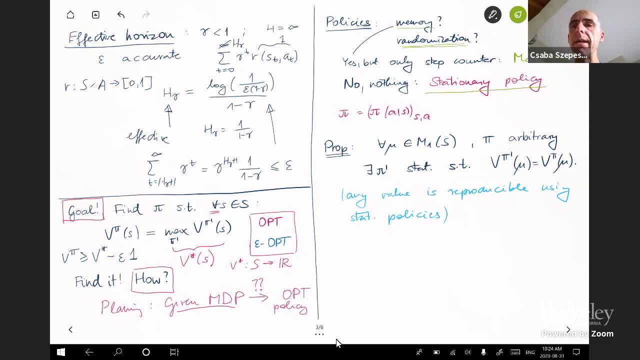 So it doesn't have any memory, So could also be called memoryless policy- Maybe that's a better name- memoryless Or pure state Or state feedback. So these are all different names that people use in different parts of the literature. 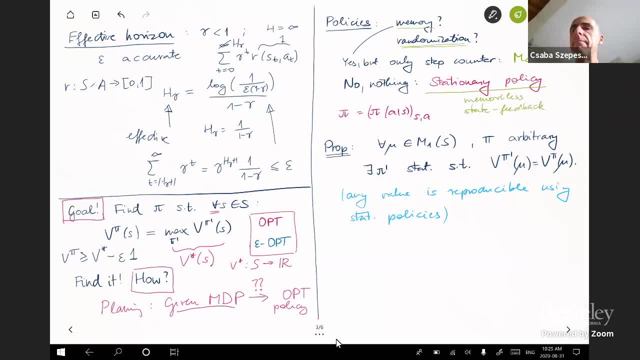 Then you arrive at stationary policies. So the claim here is that, from the perspective of finding an optimal policy, it is going to be sufficient to just focus on stationary policies. Why is that So? the reason that holds is because of this little proposition. 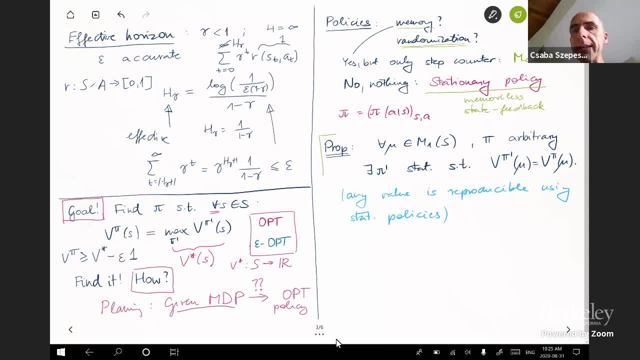 So this proposition says that if you take any distribution over the states and you take any policy- arbitrary policy- I can use memory and randomization and whatnot- then you can always find a stationary policy such that the value of the stationary policy 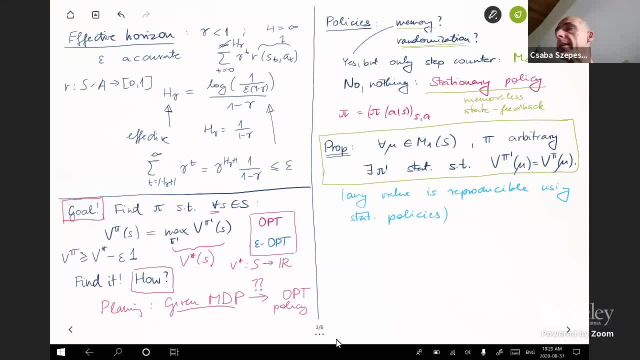 when the policy is stationary, when the policy started from this initial distribution, is the same as the value of this arbitrary other policy when it started from that distribution. So here the value is defined. Pen is misbehaving a little bit, So the value of the policy, pi, is defined as usual. 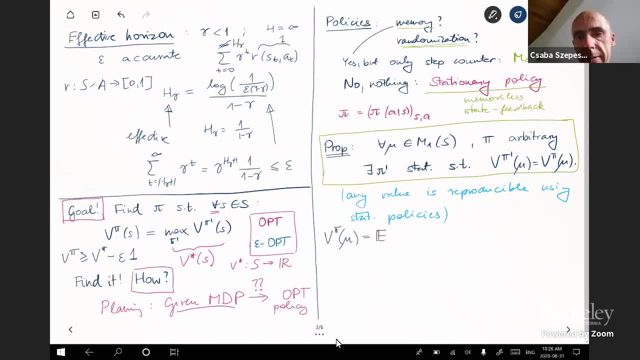 The expected value of the return And of course you can exchange. So that's a few for simplicity, that rewards are bonded, But that's always where you have food and you can exchange the you're getting it some And the expectation by the dominated convergence theorem. 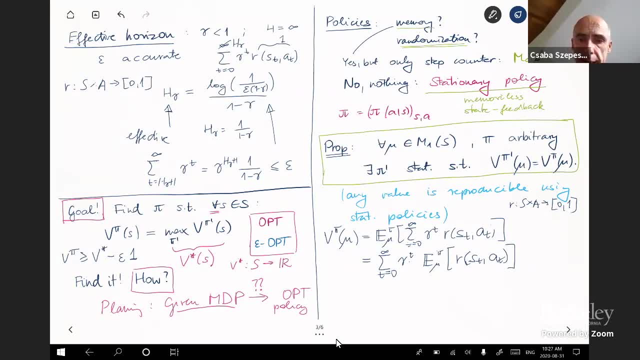 And for simplicity, let's assume that you have countable many states and actions. then you can replace this expectation by the sum. Now you take the probability that the state of time S, T is S and the action at time T is A, and just multiply. 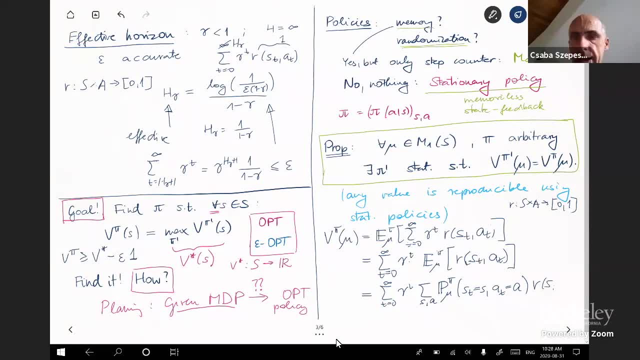 This is the individual rewards, and take the sum of all possible state action pairs, And so we can call this sorry, just do one more step, So then we can swap the sum over the state action pairs and the infinite sum And we can just call it the terms. 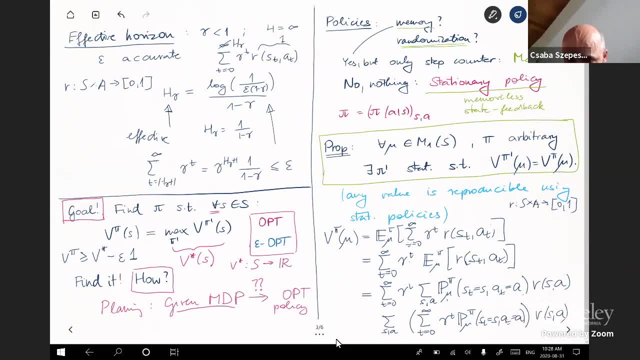 And we see that this expression arises, which I'm going to denote by mu of mu of pi at S? A. This is the definition of mu of mu of pi of S? A, And this is called the discounted occupancy measure. Let me just put this here. 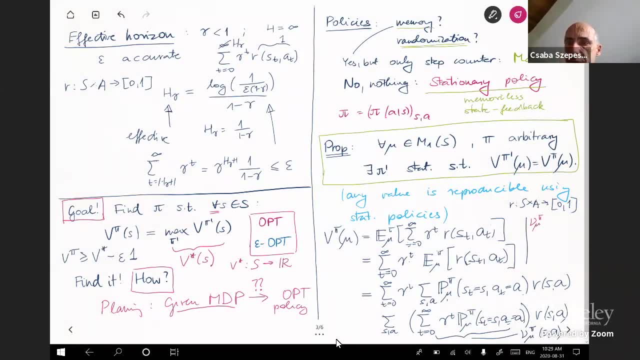 So for each state action pair we are assigning this number, which is the sum discounted sum of the probabilities of the process visiting that given state action pair at the given time step, And so this is called a discounted occupancy measure. So it Estima's a maximum. 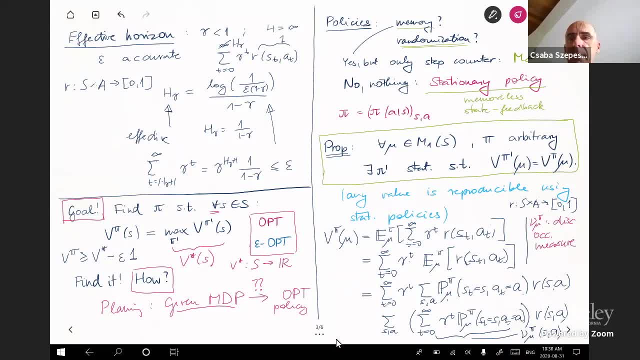 What? we're gonna give a trivial number and then we'll give a given passed logical size: disk代. Okay, So two words, this proposition. so let's recap. So we wanted it. we want to show that for an arbitrary policy it's such. this is to consider just a stationary policy. 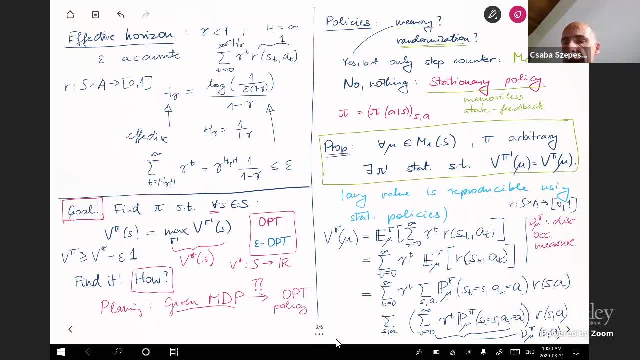 to reproduce the poises value from them. This value can be written basically as the inner product between the discounted occupancy measure, or just the occupancy measure, and the inaudible function. So you could just write this in a short form like this: If you introduce an inner product notation, 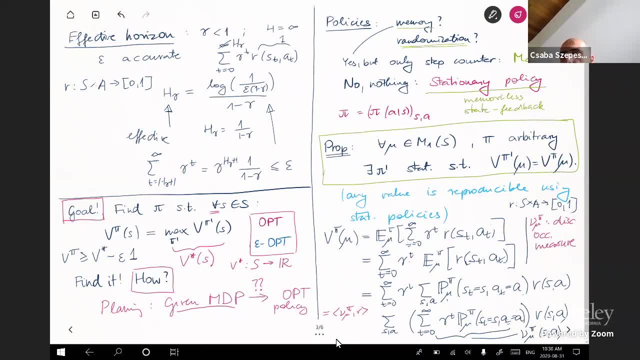 You can do this just as a big vector, and this is a big vector, So this is just an inner product between these two guys, And so, based on this, it's quite clear that a proposition would hold true. You would see that it holds true. 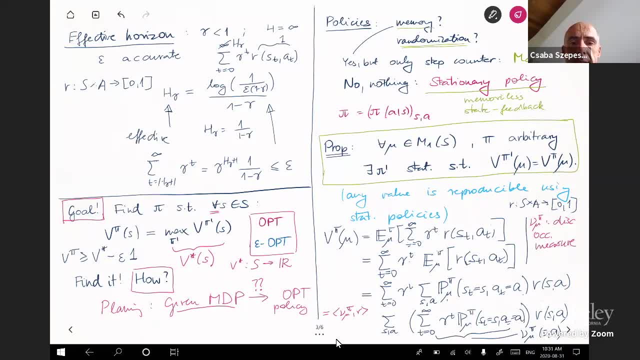 If it holds, that if I choose an arbitrary policy, pi, and I take its discounted occupancy measure, then I can reproduce this discounted occupancy measure with the help I can produce the same occupancy measure as this is the help of a stationary policy. Yes, So the proposition will be shown to be true if it holds. 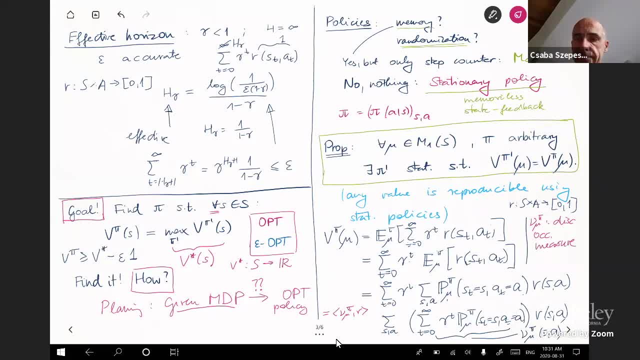 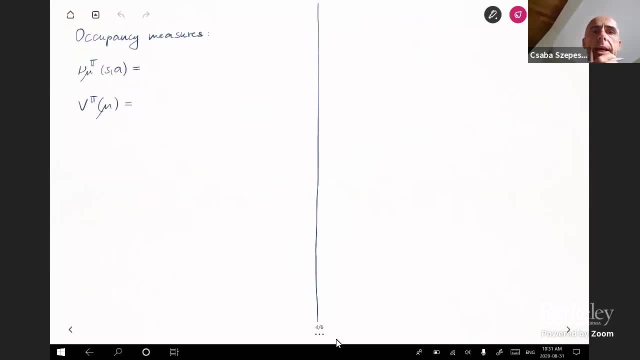 that for any- oh, I had a lot of space here- So for any policy pi. so it's enough to show that for all pi there exists a pi prime for all mu, and pi raises the pi prime such that the mu of mu of pi is equal to the mu of pi prime. 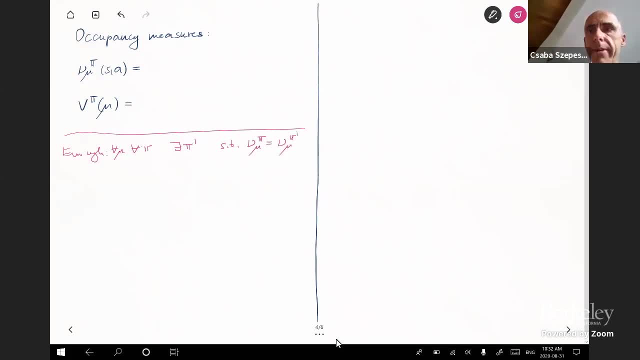 So how are we going to do this? It's a simple procedure. We are going to explicitly to be construct this pi prime and the idea is just to marginalize. So take this, so fix this arbitrary mu and fix the arbitrary pi. So this gives us this occupancy measuring mu of pi. 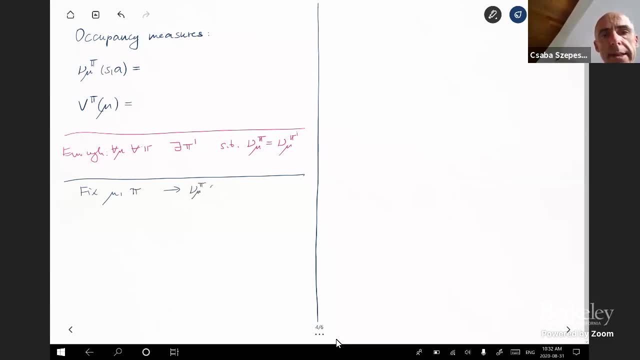 Which, if you, you know this number for every state action pair and we need to produce a stationary policy. A stationary policy is an arbitrary policy. That's because, because you know we can do it so much, We can do it so much, So we do the statistic abilities and hypotheses. 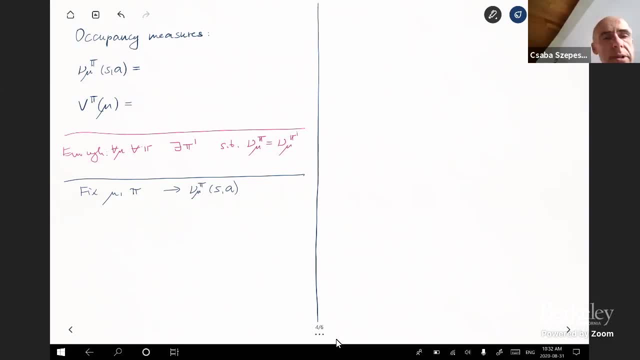 the distribution over actions given a state. So a simple way of doing this is to marginalize, and in a good way. So this is how it's going to work. So we just take this counted occupancy measure and we divide by the marginal. So mu of pi of S is going to be the sum. 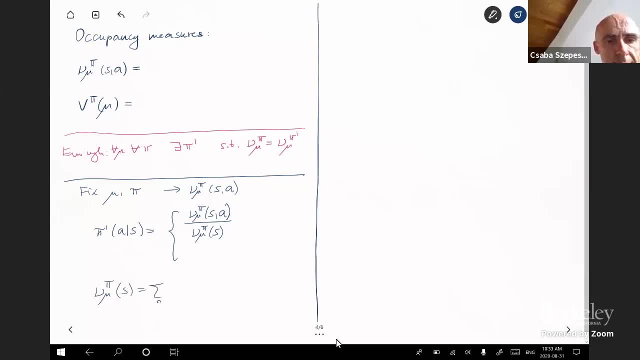 over all the actions of the same thing And if this is not zero and we assign an arbitrary distribution. if this is not zero, this happens to be zero. So this is pi naught is just an arbitrary distribution over actions. It doesn't matter what distribution you choose. 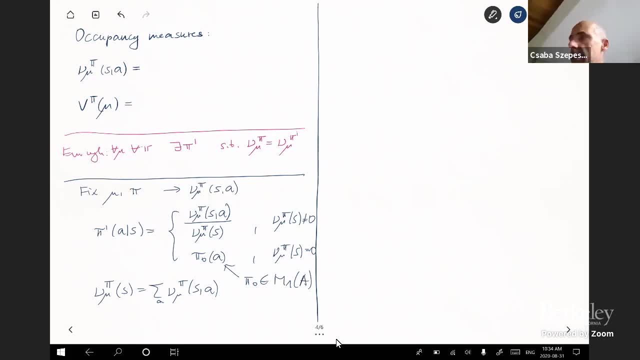 So I don't know that I should go through why this is enough. Maybe I go through why this is not just very quickly. So let's define this Markov kernel: pi of S of pi, prime of S prime. as you know, this given a state as policy. 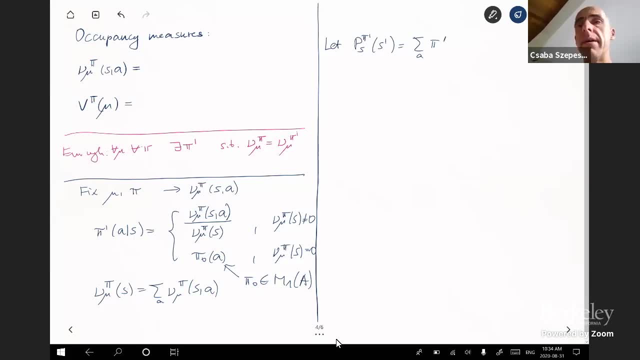 pi prime first chooses an action A with some probability, And then we are making a random transition according to the transition dynamics that we have, And so note that this can be written as the sum of because of the definition of pi prime. So just plugging in the definition of pi prime. 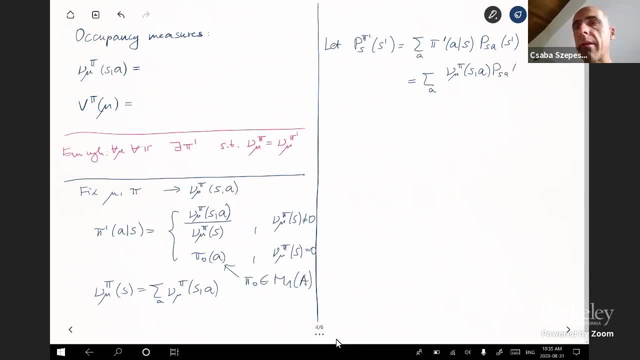 So I'm just like: this is the theory that I heard. So that's the very first thing. You know. it's a very interesting method, So this is what can be done. So what you do is you multiply it by the linear base. 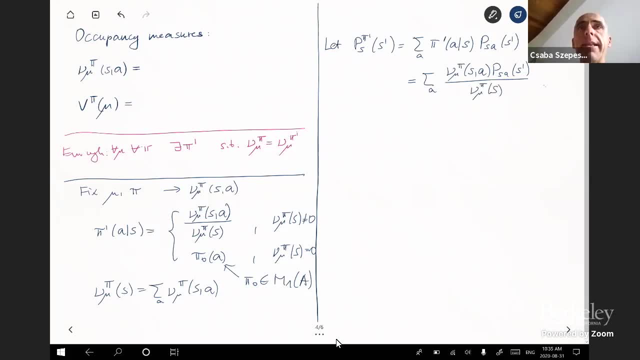 And this is how you multiply the variance. So we have the advantage over the linear base. Now what I want to do is I'm going to multiply by the linear base and then we'll have the derivative of n over n times n over n times n over n. 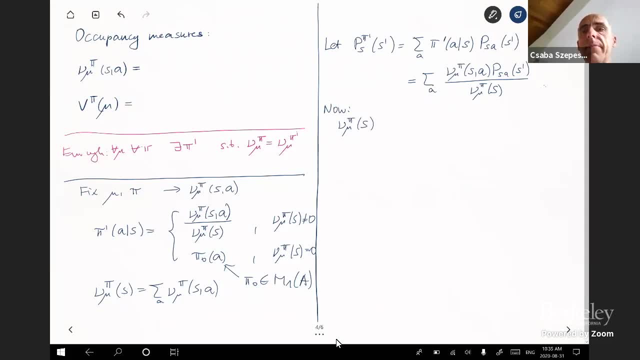 So I'm going to draw it by the linear base. So we're going to take the linear base and we're going to divide it by n over n times n over n times n. So now we have the linear base by definition, this discounted sum of visitation probabilities. 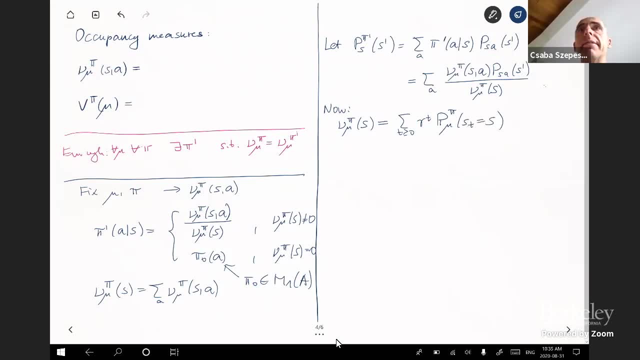 of this particular state And you can break the sum into two parts and you will see this argument many, many times. So this probability distribution, of course for t equals zero. it's mu of s, because that's your initial state distribution. 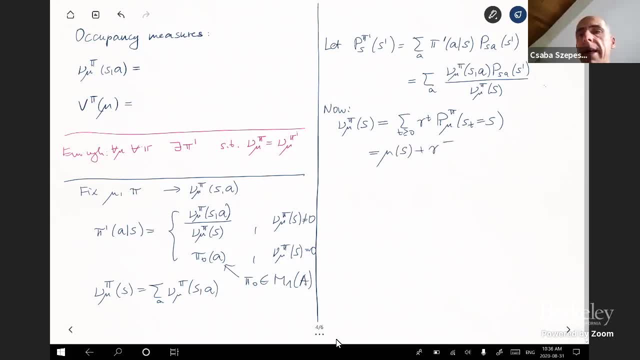 And for all the others you can just pull out a gamma and you get gamma of t plus one of p of u of pi and s, t of pi of s, And so now we're gonna use the Markov property. So just sum over s prime and a lower after that probability. 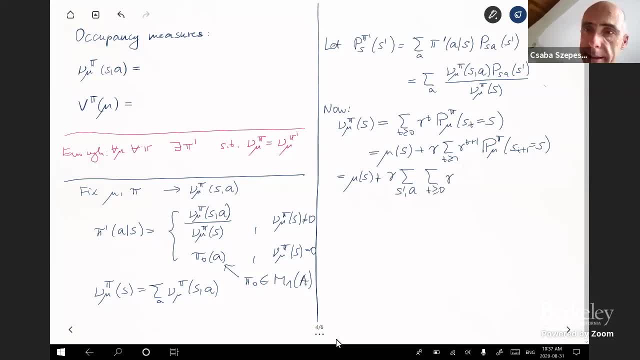 Sorry, this is just because I pulled out the gamma already, So I want to bring in the occupancy measure. That's why I'm doing this. So I write this probability, I expand it based on what the previous state action pair could have been before we arrived here. 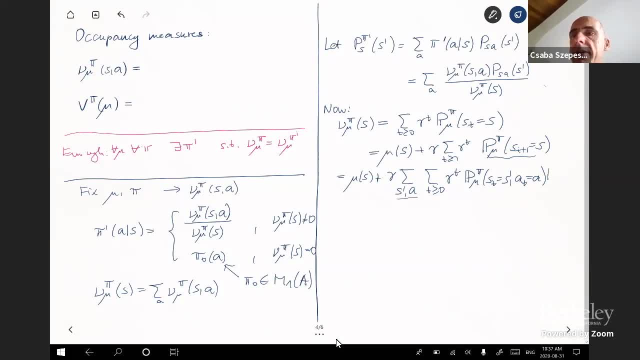 And then that introduces the Markov kernel. So we're going from s prime, S prime, using action A, to state S, And now you can see that this is just mu of pi at S prime and A, S prime and A, And now you can start to see that. 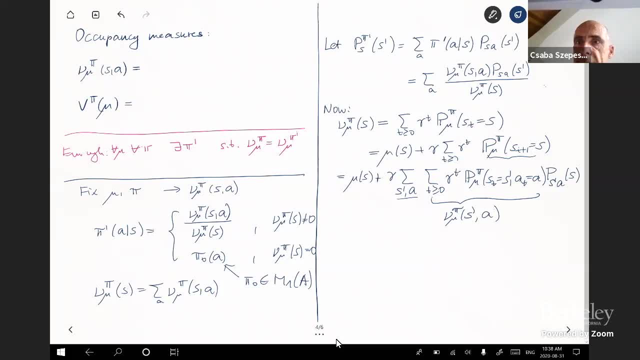 we have the same expression as S. I don't know whether it's clear, but I'm pointing. We have the same expression as here, except that S is here S prime And that S prime is S. so swap S and S. 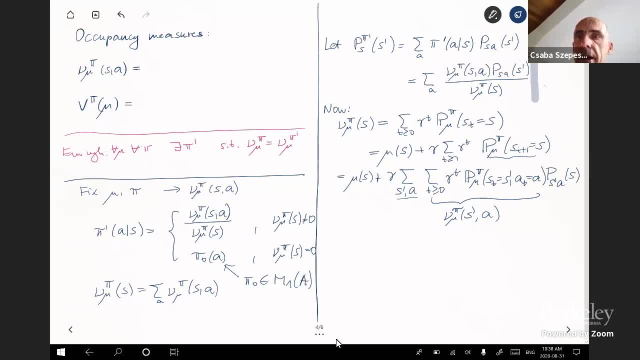 S prime. So using this, we get that this is mu S plus gamma times, sum of S prime and A of pi prime. Sorry, I need to bring in mu of pi S prime because I need to divide and multiply And then I have the sum of reactions. 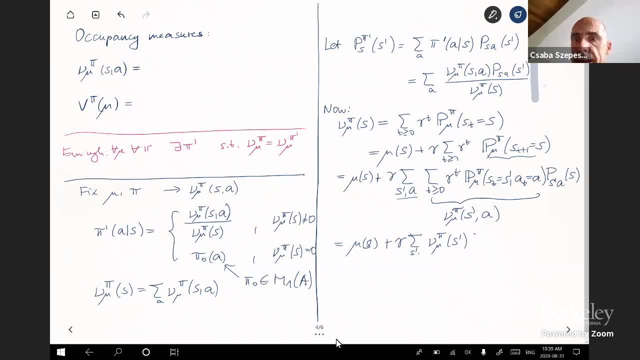 I can replace that just with this: prime S, prime A S, prime A S, prime A. And now this is nothing but the transition kernel that we introduced before. This is mu of pi, prime S, prime S, s, and with a vector notation. what we derived is that mu of mu of pi is equal to mu plus. 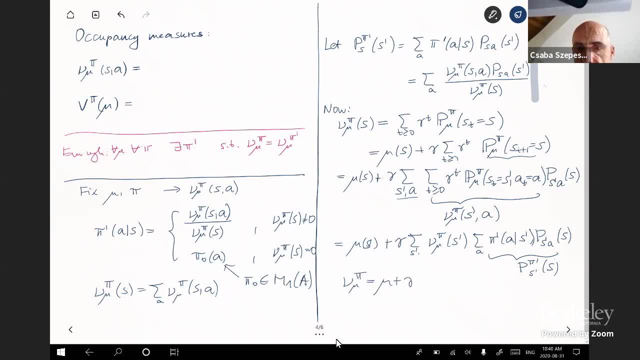 gamma times: mu of mu of pi, p of pi prime. another argument is that, uh, this equation has a unique solution in terms of uh, mu of, mu of pi and uh. by repeating this same argument, you can find that, uh, the unique solution of this equation is actually mu of mu of. 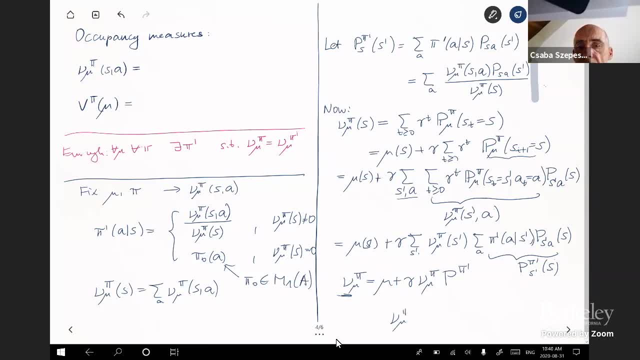 pi prime. so it follows that uh, mu of mu of pi is equal to mu of mu of pi prime. so uniqueness, this and and apply this with uh for the same reason in this pi set to pi prime, right, uh. so that shows that this shows that uh, this construction. 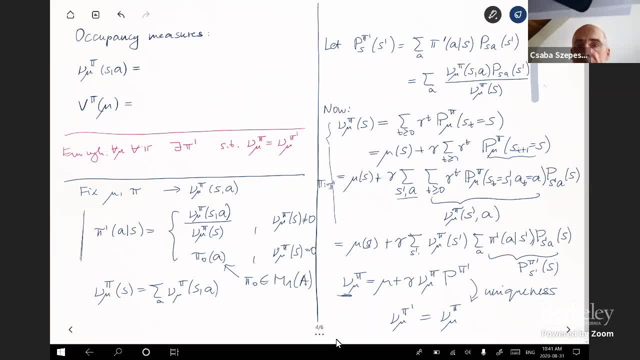 uh, does everything, uh, that we wanted. so the corollary to this- using here too much time to correlate to this- is that there exists a pi, which is a stationary policy which is optimal. so why is that? it's because, uh, we showed that stationary policies are sufficient to. 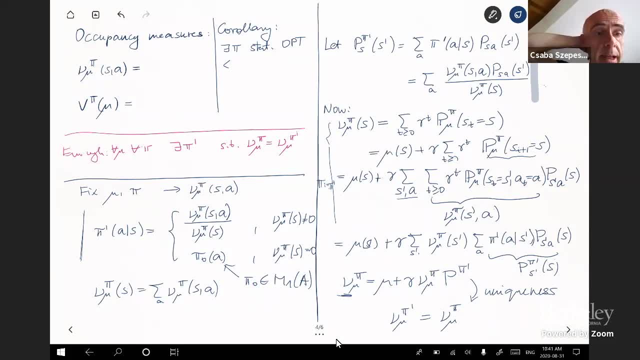 to um reproduce the values for any given initial state of any policy, and so first you can construct a policy, uh, i mean okay, so for really the existence, not absolute optimality, you need to have some uh additional um, my structure assumptions. but for example, if the state, action, space is finite, 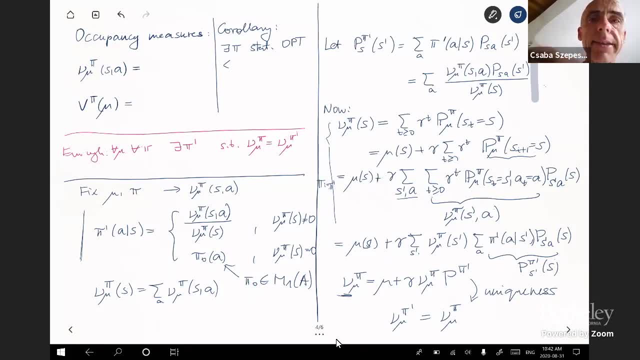 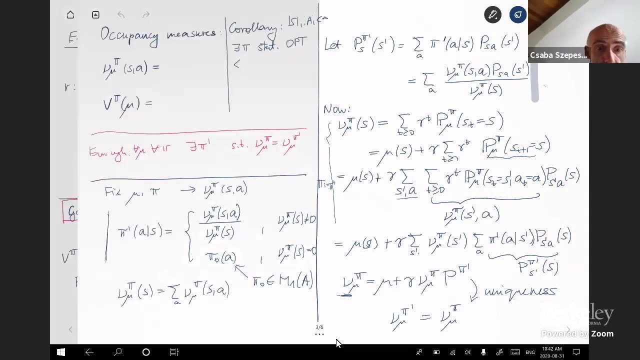 okay, so let's, let's be uh, specific, uh, state x and x is finite, uh, then you can first find a policy which is optimal, right? so the optimality definition was that the policy needs to achieve the maximum value at every state action pair if you start with an initial status. so that's, that's an v, that uh. 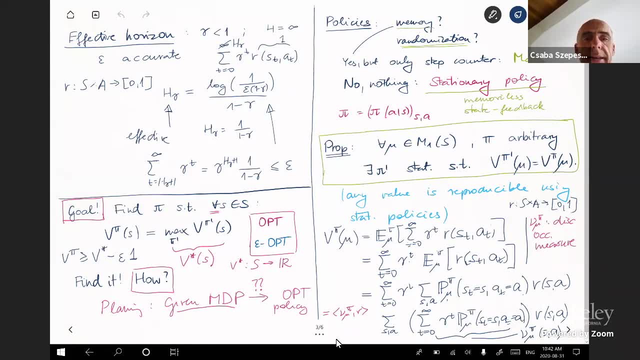 is a drop at s? uh, then you just have to maximize this, this in that product, and so you can find a policy, uh that uh really achieves that value. and that's because, uh, the space of occupancy measures- uh, it also follows from this derivation is- is a nice compact convex set uh. this you can. 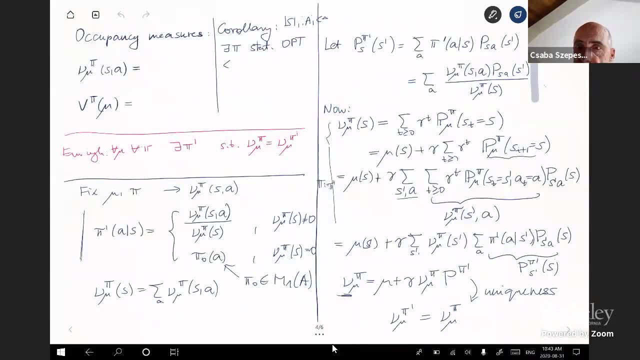 see from somewhere here in the middle, like you start here and the occupancy measure satisfies this, this activation here, so you can plug this in and cross out this mass and so that's just the linear constraint on the occupancy measure and uh, and you can show that, uh, if you have them, uh, some other constraints, no negativity. 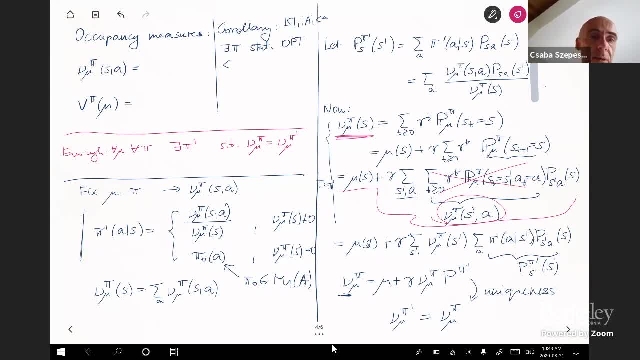 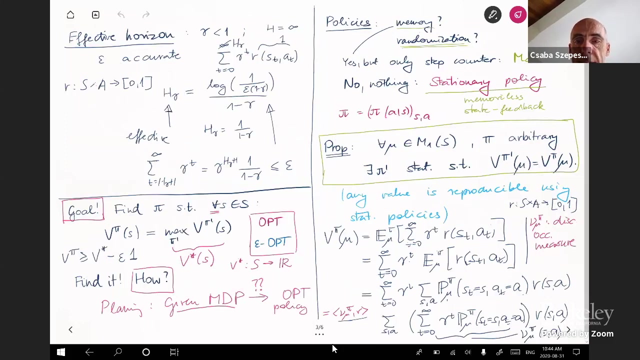 and some optimization constraints, then, uh, every element, every um measure, every uh function of state action pairs, uh that satisfies this linear constraints of the fancy measure, and and it's a nice convex, compact set. and then you can find a policy that uh, maximizes, uh, the value for a given state and uh, if, since the policies are not restricted, you can also stitch. 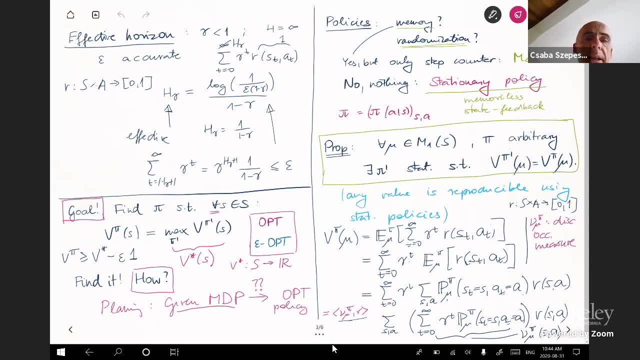 together policies and find a single policy that looks at the initial state and say that, oh like, if initial state is this, then you just use this policy, which is optimal for that initial state. you stitch the policies together because policies can remember what was the very first state. 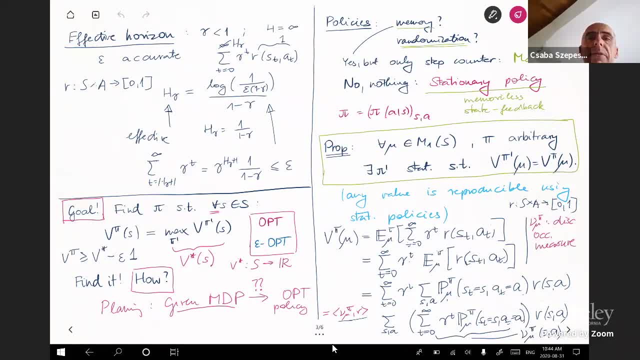 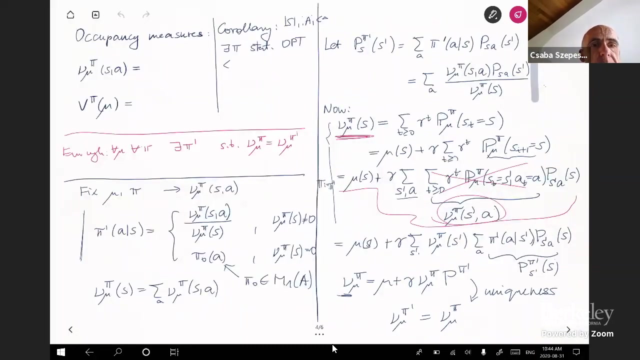 and so, this way, you arrive at the policy which is um, which uses memory, remember the very first day, and is optimal. and uh, once you have that, you can reproduce the value of this policy by a stationary policy. and and which stationary policy? well, this stationary policy doesn't depend on um, what, what the initial state the solution is going to get. it happens to be. 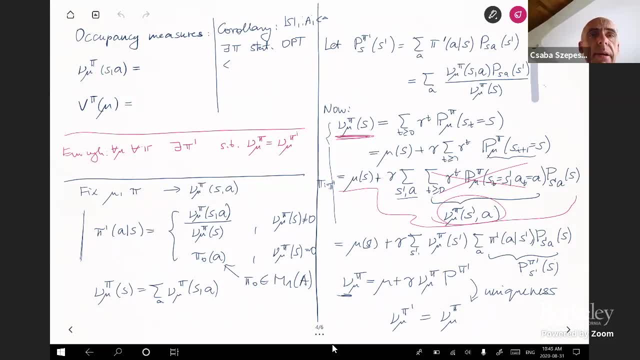 true, uh. so, uh, it follows that there exists a stationary policy which is optimal. uh, i guess, uh, maybe- maybe he's going to talk a little bit more from a different angle about this- and uh, it also follows that there exists, uh, a policy, uh, which is deterministic, uh, which is optimal. all right, uh, my time's really up, uh, so. 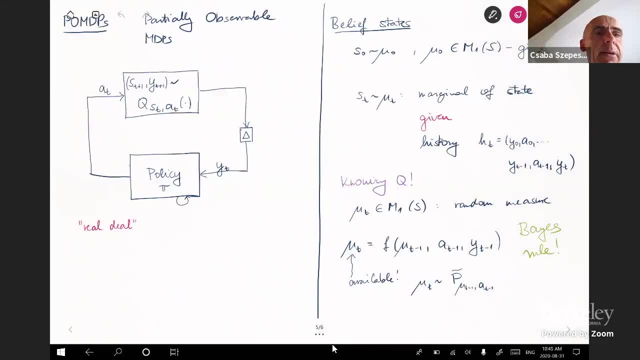 i just wanted to say a few words about partially observable mdps. uh, so, um, the previous figure showed that, uh, the controller or policy receives the state and and very often, uh, it is the case that the state- uh, which is the summary of all the past information- is not available for measurement. 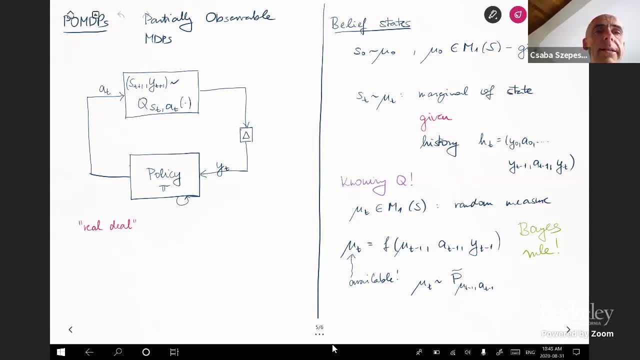 and a more general way of thinking about control systems is not to assume that the state can be observed. so still, maybe there is a state, uh, that is being updated, but instead of having a mark of kernel that, uh, it gives you an x state and then you observe the. 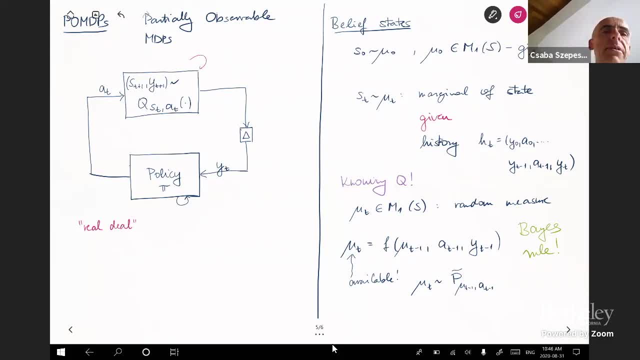 state: you have a markup kernel here, q, which gives you a pair of states and actions and states and observations. So this is next state, obviously, and this is an observation that is going to be fed to the controller. So in this case, the controller can only use the observation. 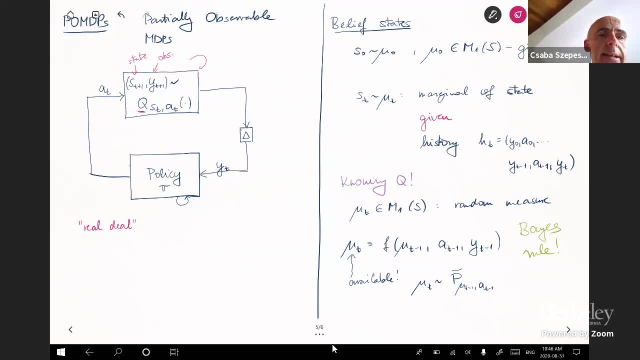 and, in a way, this is the idea. This is how, most of the time, control systems need to practice with their environments, And the question is: can you extend any of the things that we were previously said to this case? This happens to be, in a way, true. 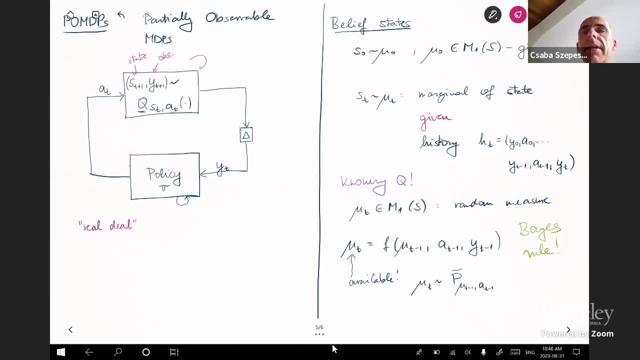 If you start with an initial state distribution- mu naught, which is known, given to you- then the marginal distribution of the state given a history at some time, step t- let's denote it by mu of t- satisfies a recursive update. 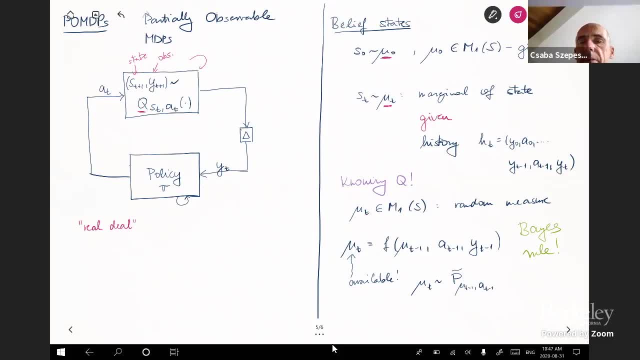 So mu of t can be seen to be computable as a function of the previous distribution, the last action and the last observation, And for this you just need to use Bayes' rule, basically, And it happens that you can also think about mu of t. 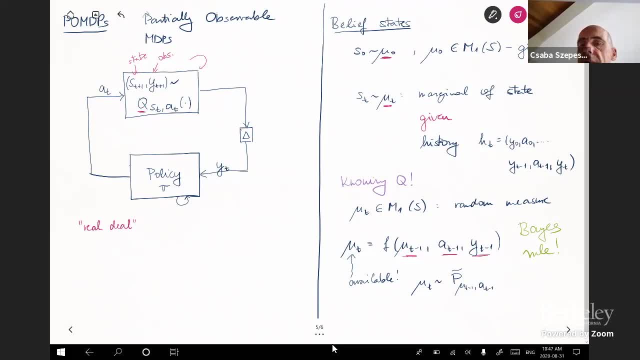 as being randomly sampled from some underlying transition kernel. So this way we're lifting the problem of computing optimal policies from policies that depend on states to policies that depend on distributions. So an optimal policy in PAMDPs would keep track of the distribution. 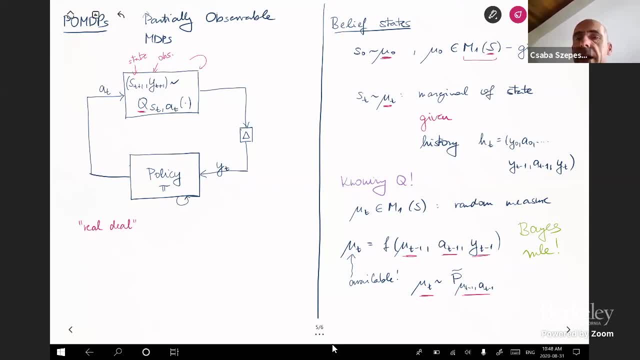 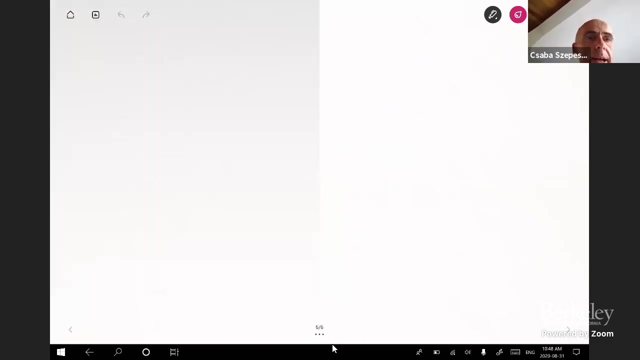 uh, this ronal measure, this belief, uh, state or belief distribution over the state space, and i would use that as a summary and then you can try to to generalize: uh, resides the constructions and so forth. all right, um, so i think that with that, uh, i'm done. uh, let me see whether 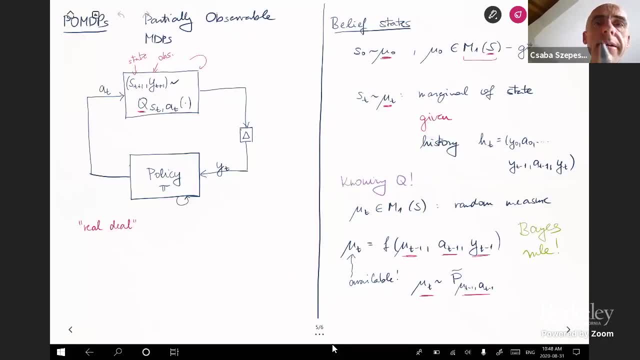 well, i used a lot of time, so i should just wrap up. oh, what happens, uh uh, when the reward is not bounded? uh well, you need all kind of regularity conditions, or you could have costs, even, um- in order to be able to define values, and some policies may not. 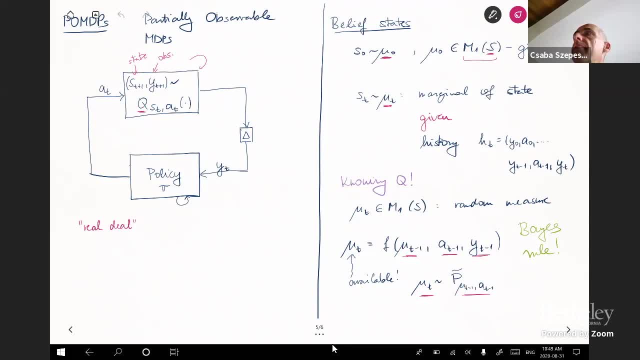 have values. the same problems happen when you don't use discounting uh and uh. in this case, people assume more kind of regularity conditions so that to make sure that uh, even uh- you know the notion of optimal policies is well defined. um, all right, maybe are you around. 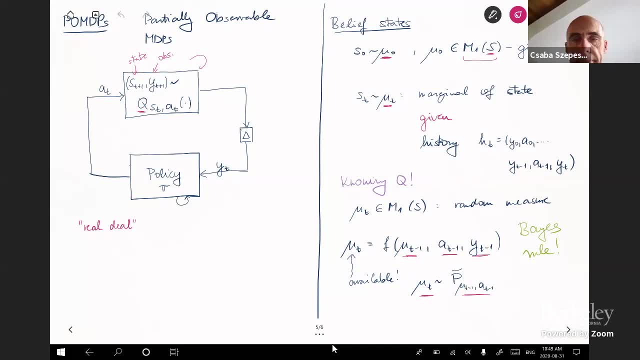 hello, yes, okay, sorry. uh. so we ran a little bit over time, sorry about that. um, that's all right. i'll try to be very high level. okay, let me see it is yours. i don't think you want to um much screen. i, yeah, i can share my screen if you're sharing yours, okay. 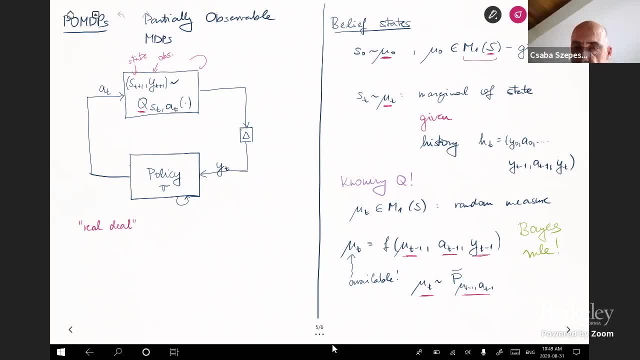 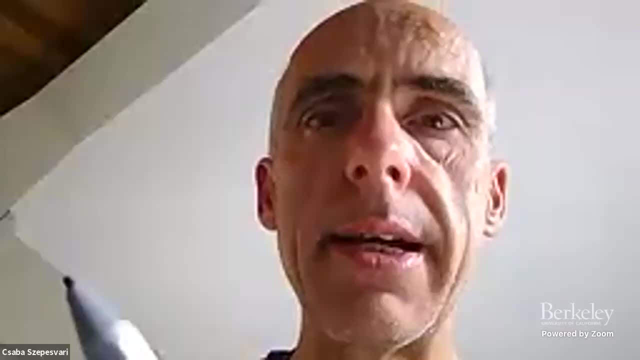 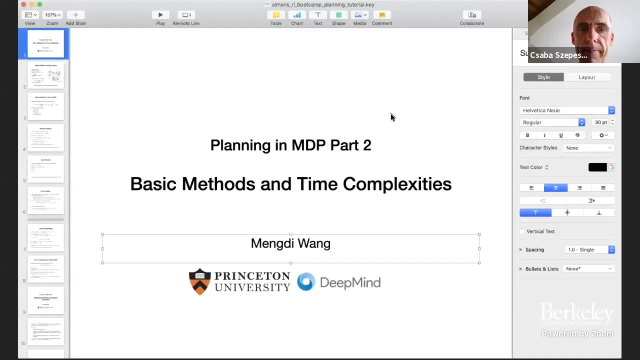 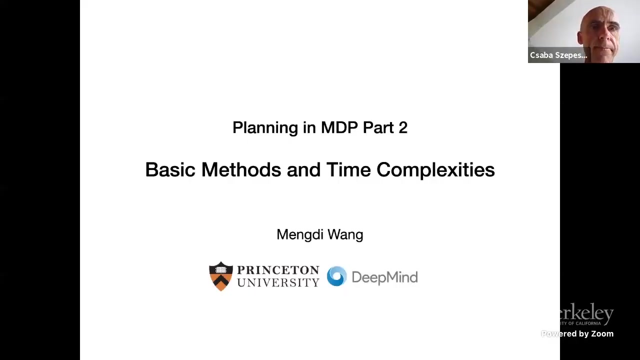 how do i understand about sharing? okay, stop, okay, i think it's okay. does it work? i think so, yes, okay, um, so next. so we want to talk about the very basic methods and complexity results for planning in markov decision processes and like, as trevor has, 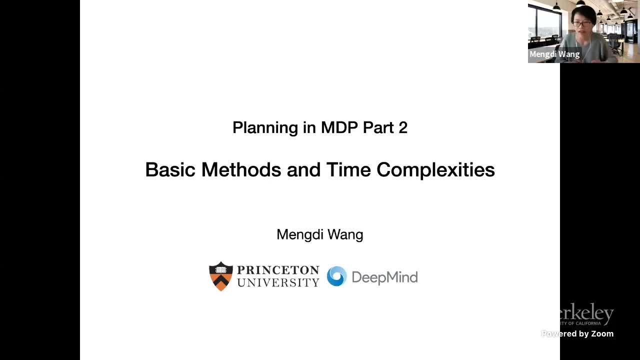 mentioned, like reinforce learning, is a very broad problem and there are many problems that are extremely hard, like partial observable markov decision process and like the other problems that are more complex, and also for continuous problems with unbounded space. usually the problems become harder and there's another like nuances, so to talk about complexities again, so we want to focus on the. 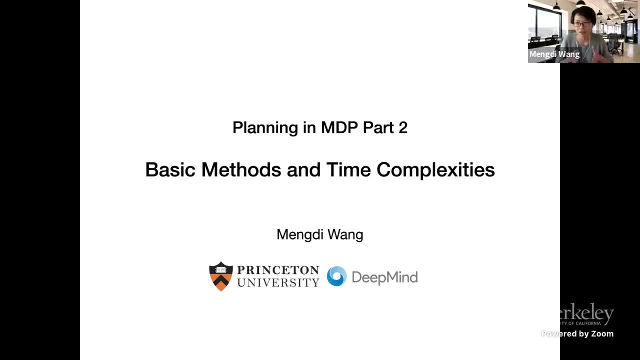 simplest: finite state, finite action, markov design process and assuming everything is bounded. so this is a notation we are going to use. we have a finite set of states, a finite set of actions. Each state of action, we have a reward, which is a scalar. 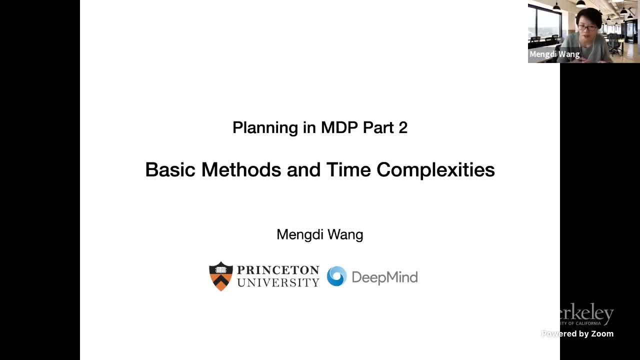 And we have a collection of state action to state transition probabilities. So all of those are input to the algorithm And based on those we're trying to solve the optimization problem and find the optimal policy that maximizes the cumulative discounted sum of rewards. 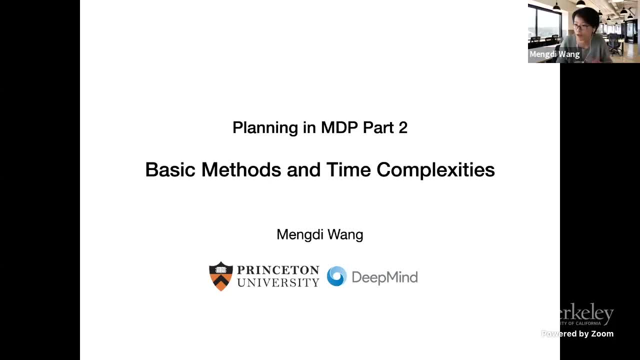 Okay. so this is just a statement of the problem. We have already simplified it to the most. So no unboundedness, no partial, everything finite. Okay, so usually we call this tabular Markov decision process, because we don't really have much structural information. 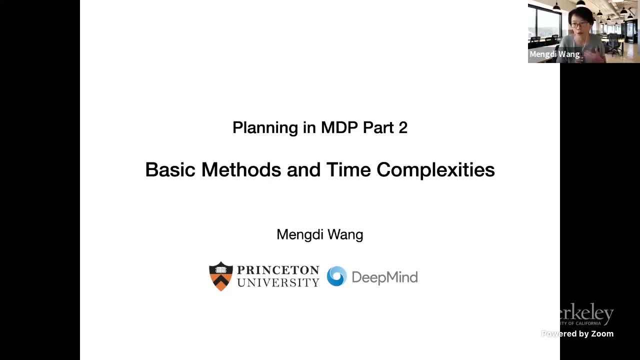 or additional prior knowledge here, just a discrete computational problem. Okay, so what are the basic methods? So first, whenever we talk about solving Markov decision problems, we usually always write down the optimality condition, which is known as the Bellman equation. 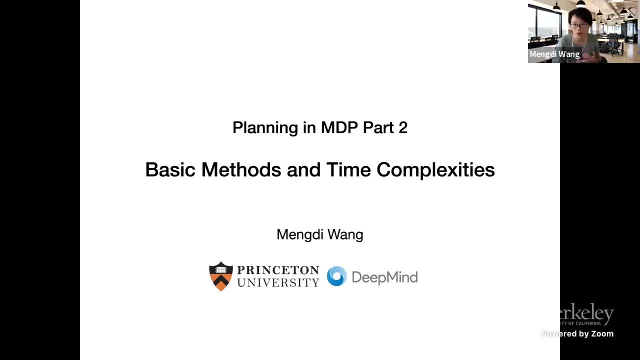 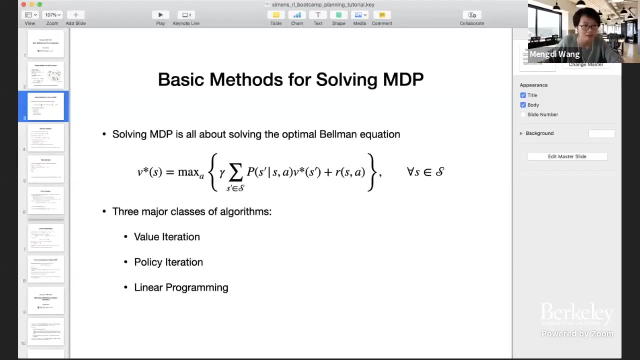 or the optimal Bellman equation, So the optimal value function, which we call the V star. Maybe your slide is stuck at the title slide. Sorry, I think that happened to me a lot. I have to, Yeah, stop the presentation mode. 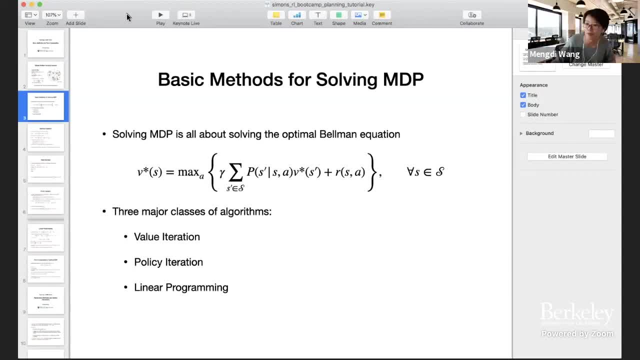 Does it work now? Hello, Yes, I see the Bellman equation, yes, Okay. yeah, So I was talking about the basic notations and now the Bellman equation. Okay, so we want to compute the optimal value, function and in the discrete case, 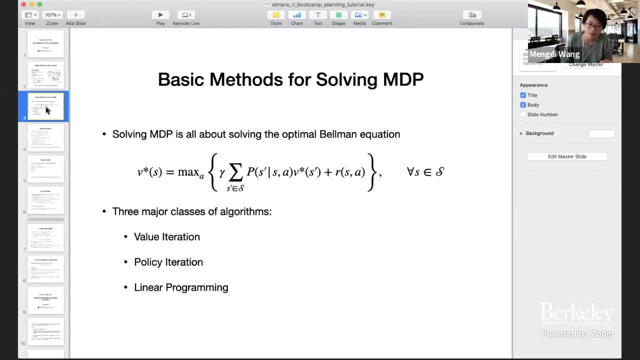 the optimal value function is just a vector and the dimension of the vector V star is S, The number of states. Okay, so there are three major classes of deterministic algorithms, but they turn out to be the foundation to many learning algorithms, So we'll just go over them one by one, but very briefly. 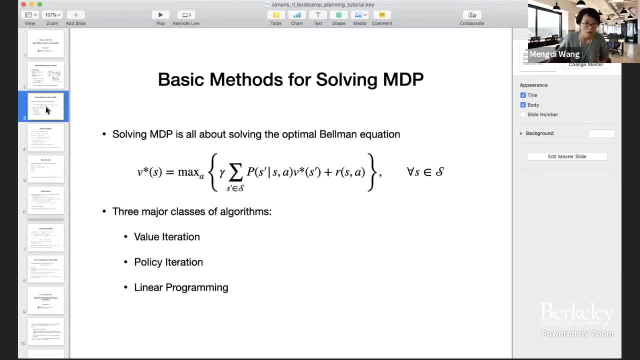 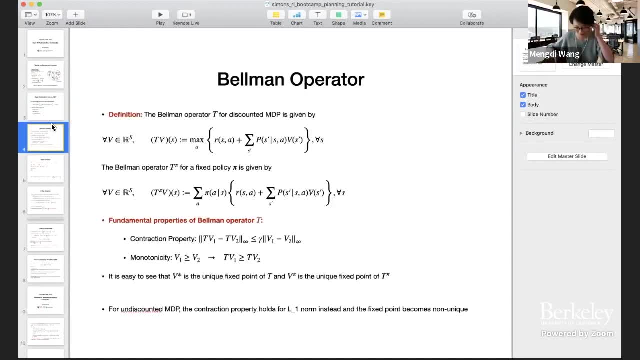 So the first one, actually, before we go over them, yeah, we need to introduce a notation called the Bellman operator. So the Bellman operator comes from the Bellman equation here. So the Bellman operator is going to be the operator. 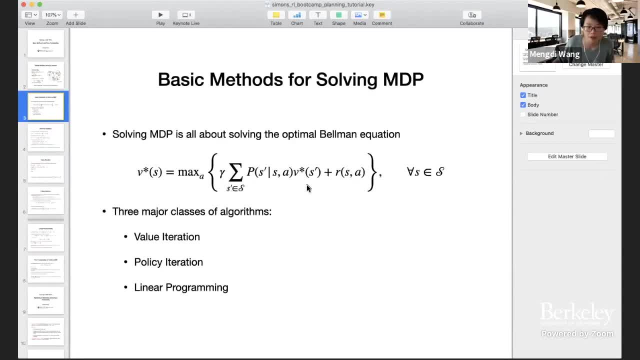 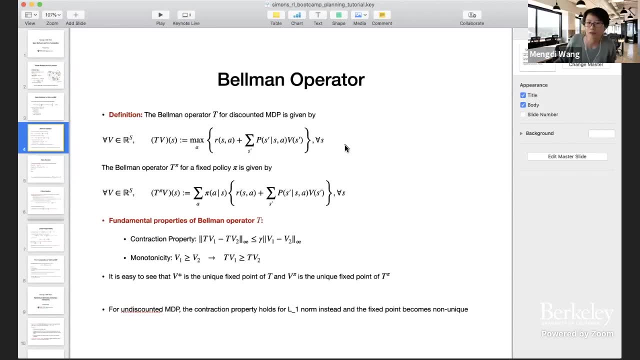 that maps some value function here to the left-hand side. So it's defined in this way. So we can apply the Bellman operator T to any value function and it will work in a way as if it is doing, you know, a little bit of work. 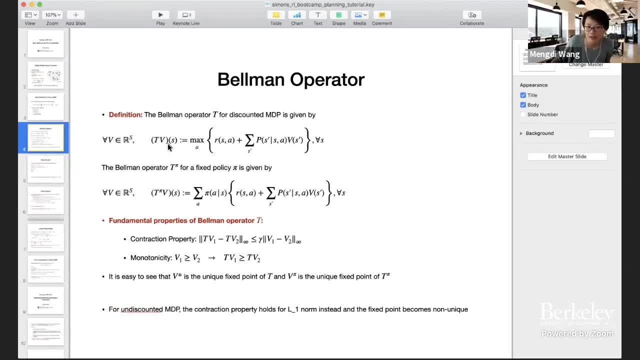 So we can apply the Bellman operator T to any value function And it will work in a way as if it is doing something. So we can apply the Bellman operator T to any value function. So we can apply the Bellman operator T to any value function. 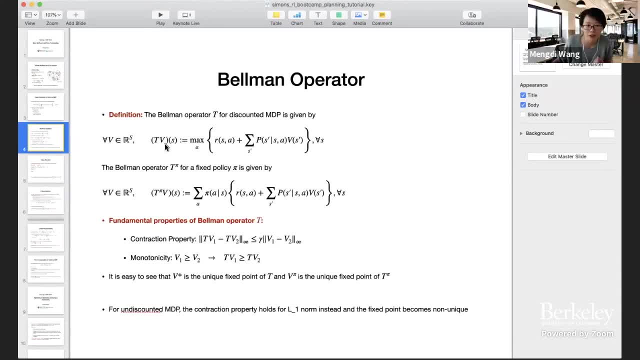 Basically, guys, this is just a one-step look ahead, basically by treating this v as the value function and that step and try to compute what's a better value function at a current stage. what's a better value function at a current stage? 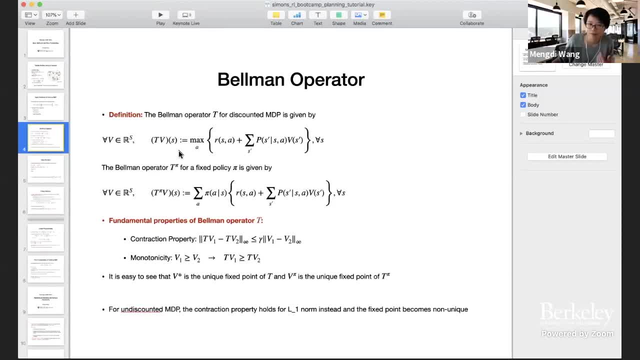 Okay and know that this is definitely a nonlinear operator And we also need notations for the Bellman operator we caught or a fixed policy. So if we fix the policy, then this Bellman operator is really just a linear operator. We simply try to evaluate the expectation of future value. 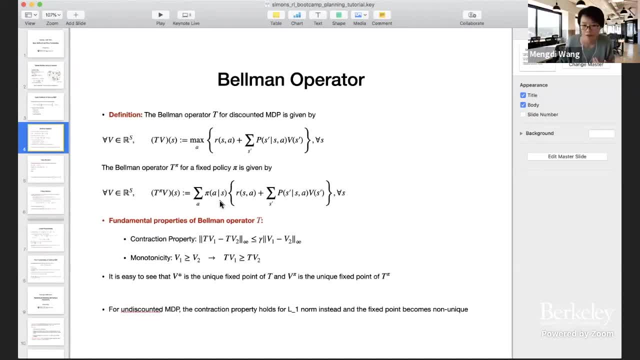 by using the probability for choosing actions based on the policy and also by using this V function as the next step value function. Okay, so the Bellman operator has a few very elegant and fundamental properties that are basically the key to a lot of analysis. 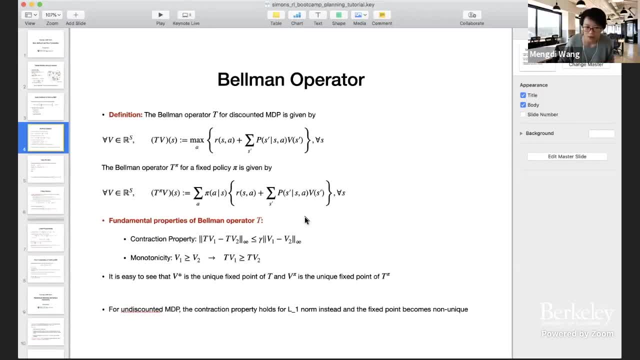 So the first property is the contraction property. Wait a minute, my apologies, I think I missed the discount factor gamma here and here We need to have discount factors, okay. So once we are talking about discounted Markov decision process with gamma between zero and one. 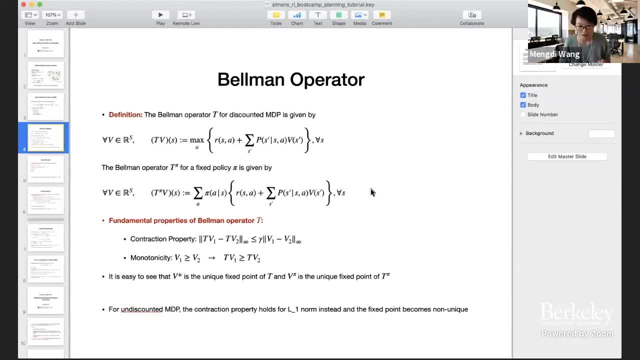 so it's pretty easy to prove that the Bellman operator is strictly contractive With respect to the L infinity norm and the modulus of contraction is bounded by gamma, the discount factor. Okay, so we don't have time to prove it now. 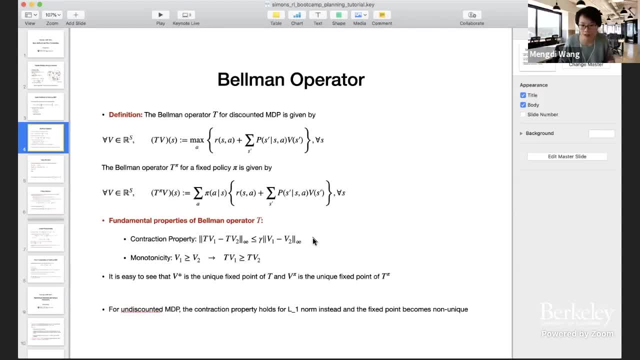 but it's really an easy exercise. Another important property is that the Bellman operator is monotone, meaning that if we start with two different functions- V1 and V2, and so V1 is point wisely greater than or equal to V2.. 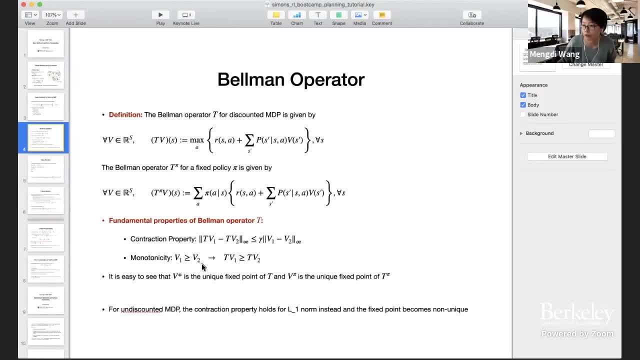 And after we apply the Bellman operator T to either, to both V1 and V2, this relation still holds. So monotonicity in value function is going to be preserved after applying Bellman operator. Okay, so, based on the two properties, 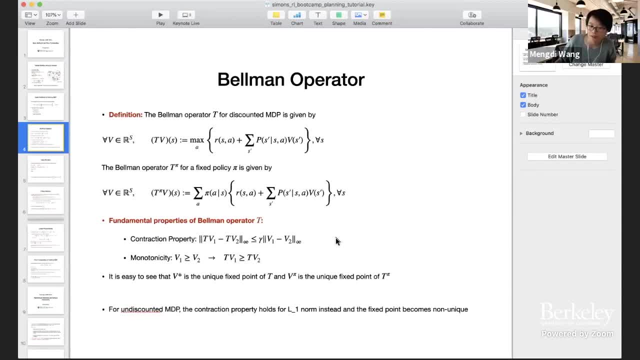 we can see that Bellman operators are very nicely behaved And also it's easy to show that the optimal value function V star is the unique fixed point of the Bellman operator And the value function for fixed policy is the unique fixed point for the Bellman operator T pi. 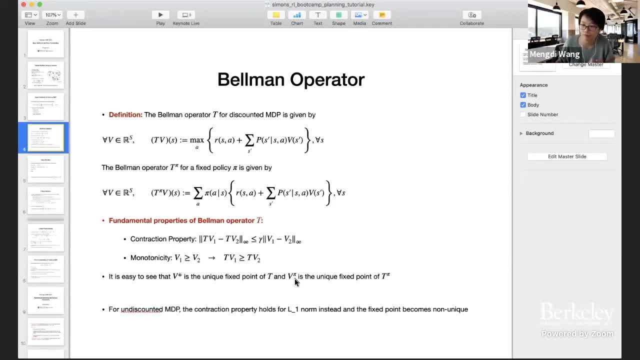 Okay, so those are very basic properties, But we do know that. but especially this contraction property heavily relies on the fact that we have a discount factor. So in some way like the process, the process always returns to some dummy state with probability one minus gamma. 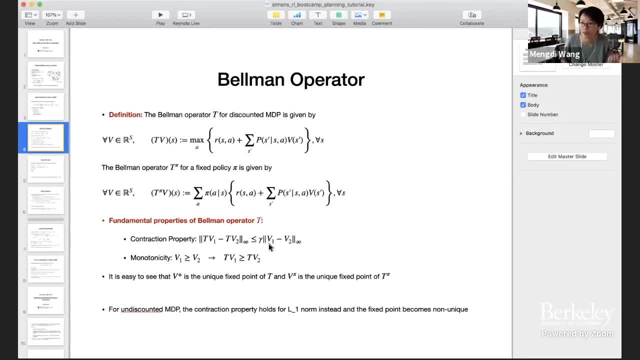 So we can think about in a by using with that. So somehow the process always return to a fixed point. That's why we have contraction. But if we don't have a discount factor, if we talk about undiscounted, infinite horizon, MDT. 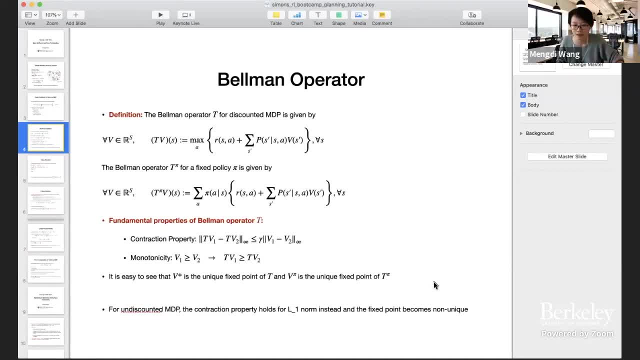 then the property becomes tricky And one can show that this property no longer holds for L infinity norm but holds for a variant of L1 norm. And there's another story, a longer story there, which I won't be able to tell today. 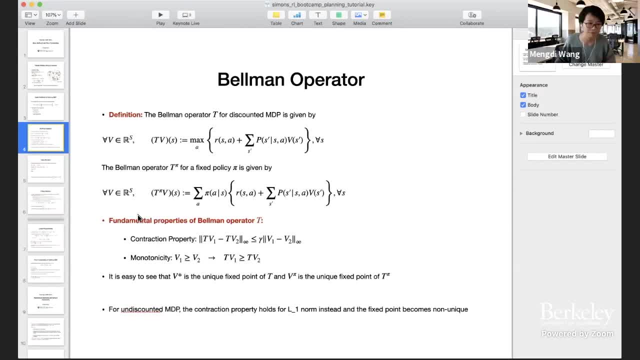 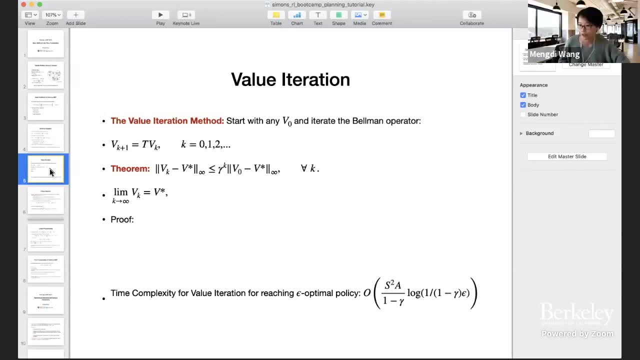 Okay, So the first, very basic algorithm is called value equation. So the algorithm is extremely simple. It basically says that we start with any V zero, any vector of dimension S, and then we just apply the Bellman operator T to that vector over and over. 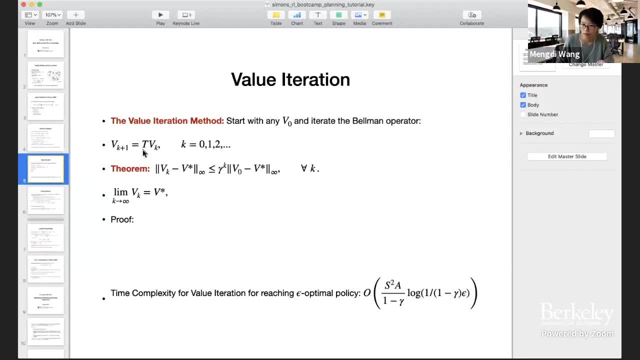 So this is called value equation, but this is really just another way of freezing dynamic programming. We're just doing backward induction, Okay, And it's about the value equation. A very basic result is: the value equation converges exponentially in L infinity norm. 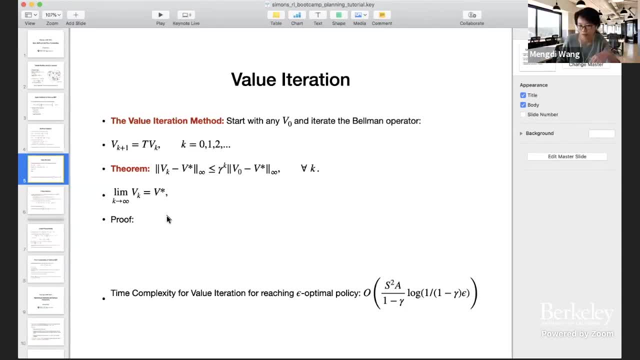 And this is a simple corollary from the contraction property of the Bellman operator. So basically, as long as we're iterating the Bellman operator, our value functions are going to converge very fast to the optimal value And similarly we can always derive the policy. 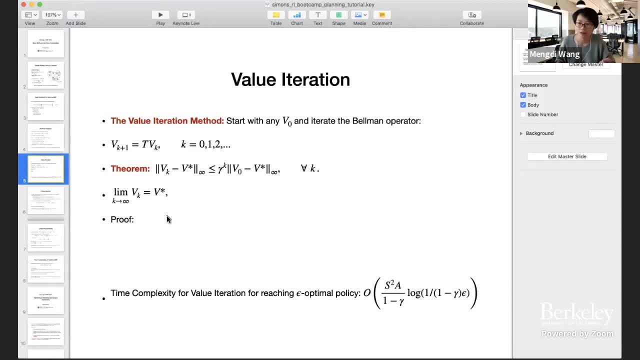 from the value function and the policy will converge to the optimal policy. Okay, So if we try to do some final calculation to calculate all the arithmetic operations needed in applying each value equation, So we can show that The runtime complexity for value equation is the following: 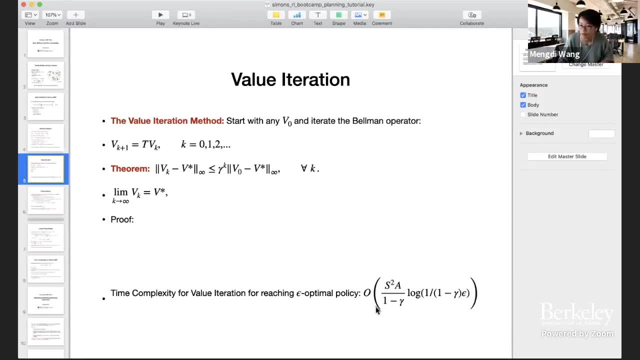 So it's of the order S squared to A. So S squared times, A is really the size of the transition matrix. So it's really the size of the input. So this time complexity is linear to the input size. And also if our discount factor is very close to one. 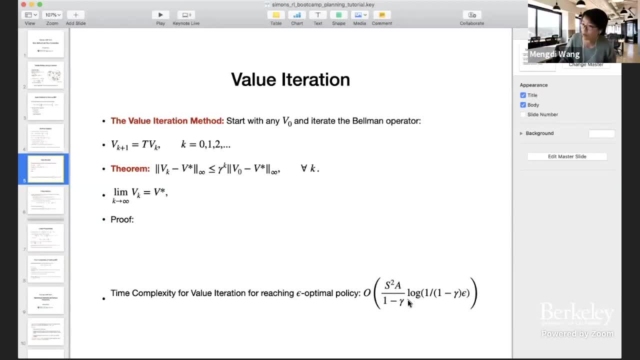 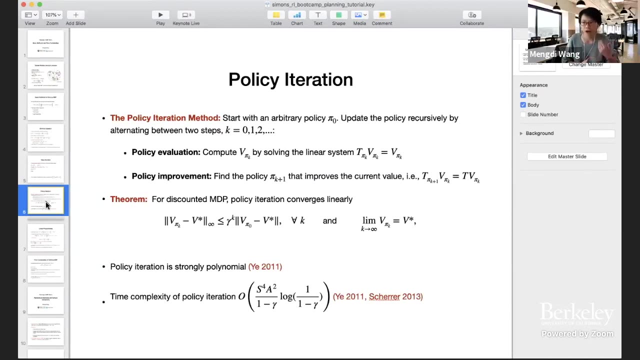 then the convergence rate will be slowed down. Okay, So a slightly more complicated algorithm is known as the policy equation. So instead of iterating Bellman operator in the value space, we try to do that in the policy space. Okay, So again we start with an arbitrary policy pi zero. 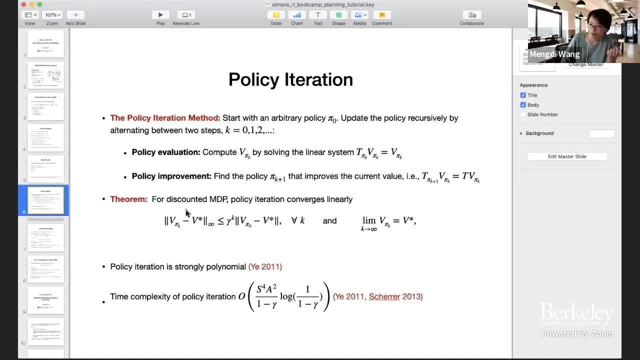 but we'll try to improve it incrementally. So to improve our policy, we always try to evaluate it first, Meaning that we want to first evaluate it first. So we first compute the value function corresponding to that policy, which is equivalent to solving a linear system of equations. 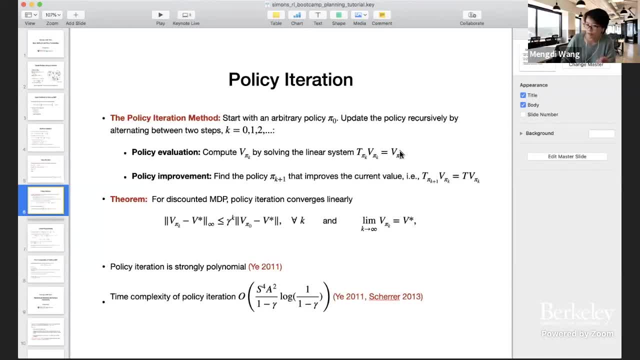 But we write it abstractly. at this T pi, K times, I would say T pi, V pi equals V pi. We are trying to solve this equation, Okay. So once we solve this equation, we obtain the value of the policy: pi K. 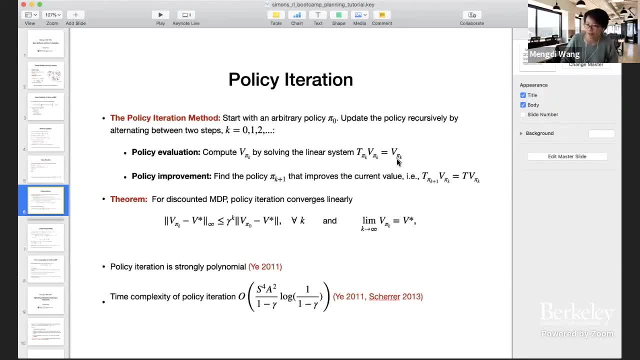 We try to improve it by basically by again doing once again one step value equation or one step look ahead. So we're trying to find this new policy, pi K plus one, such that by applying this policy for one step, we're actually doing the optimal Bellman operator. 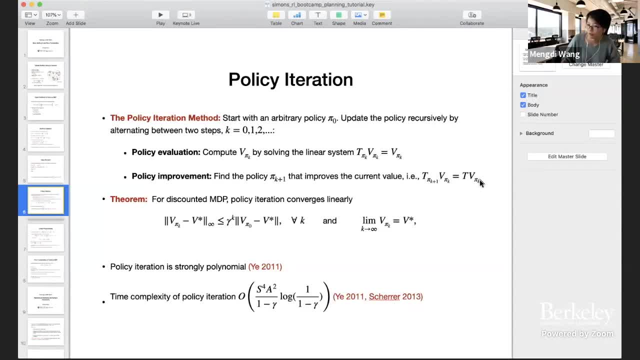 We're actually applying. it's actually equivalent to applying the optimal Bellman operator. Okay, And in a way that's similar to the proof of value equation, but slightly more complicated, One can show that a policy equation also converges linearly and the modulus of contraction. 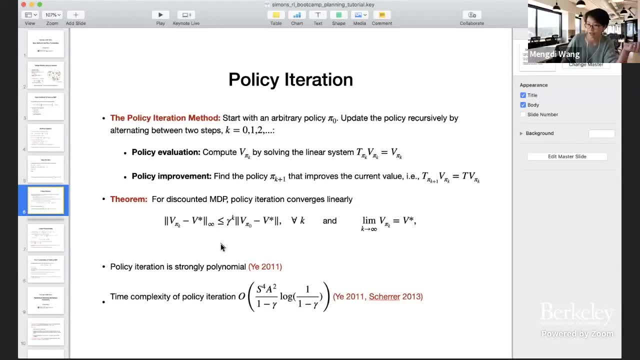 is again determined by the discount factor, And for undiscounted problem there's again a longer story which we don't tell today. So why do we care about policy equation? It looks like it's more complicated than value equation, right? 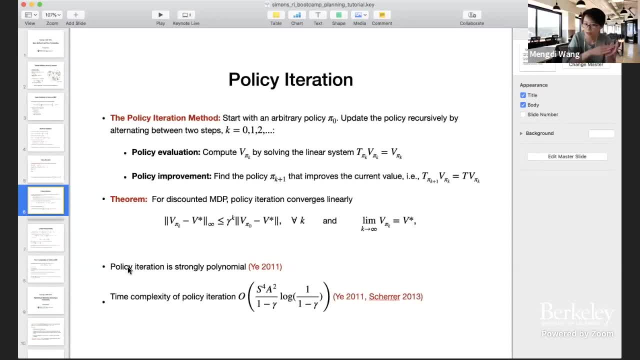 So what happens is one: the algorithm is iterating over the space of policies. The space of policies is in some way a smaller space than a space of value functions, And there are some subtle difference. For example, it's known that policy equation 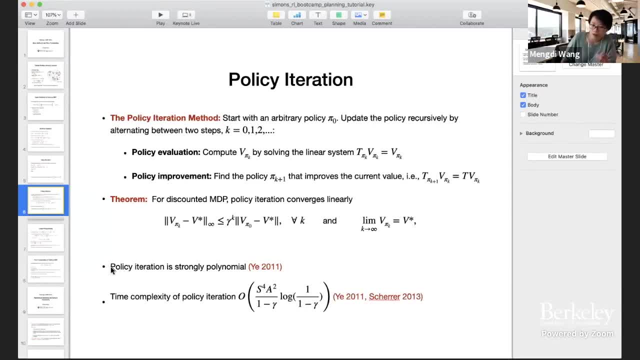 is strongly polynomial, but value equation is actually not. But, however, if we just try to implement policy equation in a straightforward way with just a regular equation solver, we call that. whenever we try to policy evaluation, we need a linear system solver. 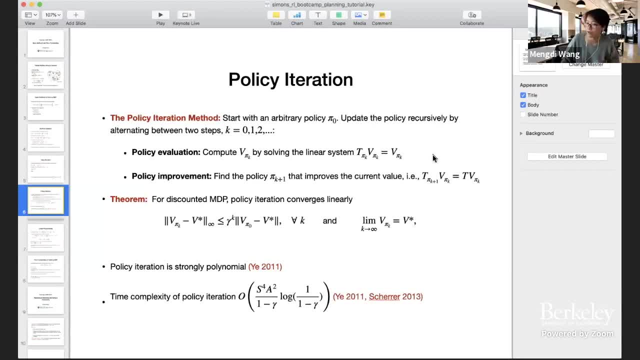 So if we just use a naive solver- we need a linear system solver- The complexity won't be too good, So we actually get quadratic complexity with respect to the input size. Okay, So that's the second approach, And the third approach is quite different. 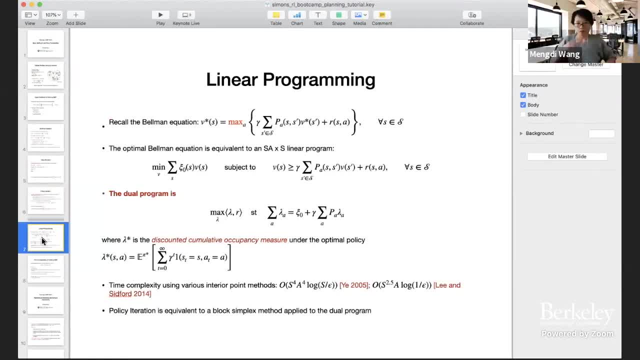 from the first two. So again we call that we're trying to solve the Bellman equation. But now, instead of trying to utilize properties of this C operator, we may equivalently rewrite the Bellman equation into a linear program. Basically, we're trying to say that: 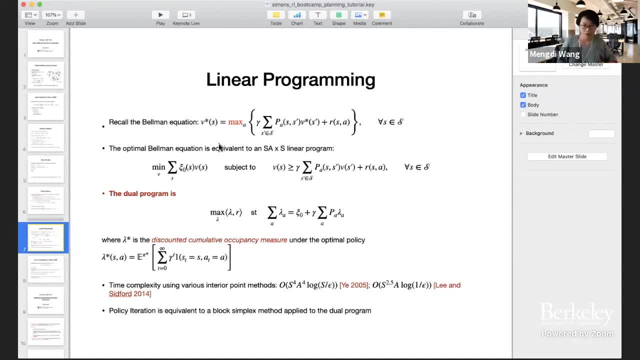 hey, we're trying to find this value function such that left-hand side of the Bellman equation is always greater than or equal to the right-hand side, And then we'll try to lower the left-hand side. So that's the intuition, And this requires a little bit of proof. 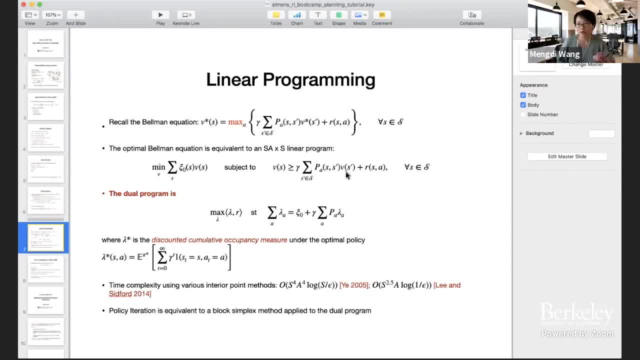 which is again a very nice exercise. Okay, So if we can write the Bellman equation into a linear program, it's going to be a linear program of dimension S, times A times S, So it's going to be a big linear program. 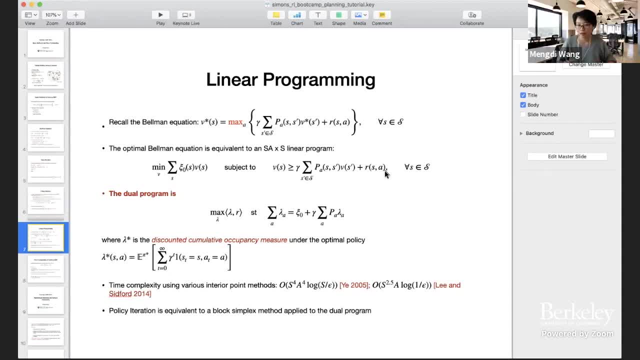 So what's interesting is we can look at the dual of this linear program. So this is like the linear program in the space of value functions, Right. But if we try to write it as dual, we're going to associate the constraints with Lagrangian multipliers. 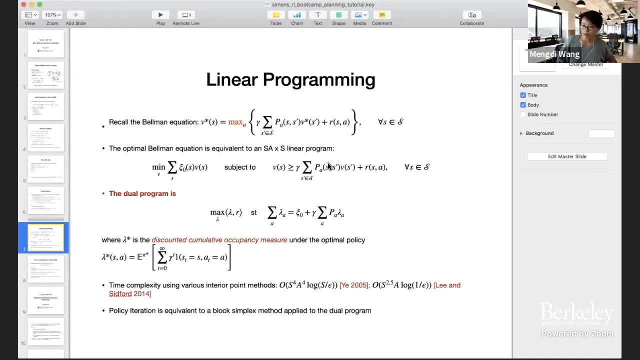 And the dual program has a very interesting interpretation. So the dual variables. we call it lambda. Okay, So it turns out that the optimal dual variable in the linear program corresponds to the discounted augmented measure under the optimal policy. So in some way lambda star tells us about. 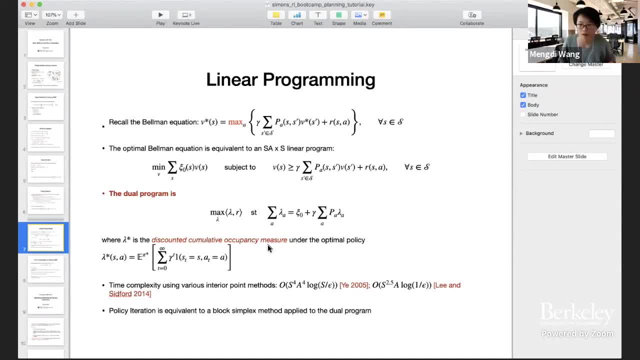 some long-term stationary state action distribution when a good policy is chosen. And if we try to interpret the dual LP, we can see that. let's look at the constraint first. This is a linear constraint and this constraint is equivalent to requiring that. 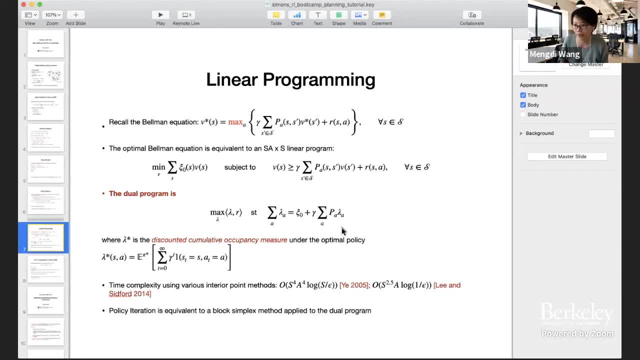 this lambda is the occupancy measure corresponding to some policy. Okay, so now we're searching in the space of occupancy measures that are possible under this MDP, And within all such occupancy measures we try to find the one such that we maximize its inner product with the reward. 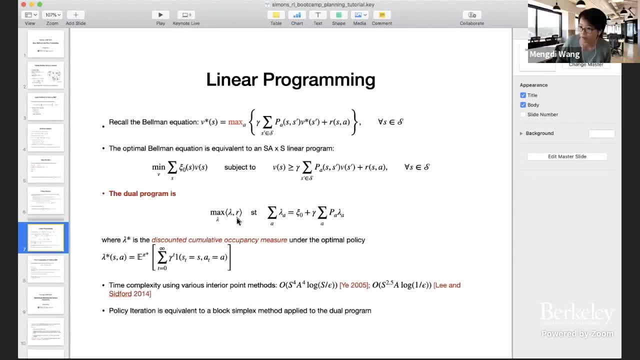 So the inner product between an occupancy measure and a reward is exactly the value function. So basically, this says that we are searching, we're optimizing over the space of attainable occupancy measures directly, And that's the dual problem. Okay, so if we think about this problem purely as 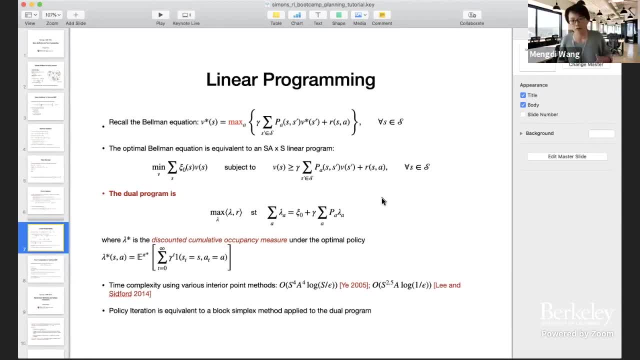 a linear program and we try to use the best interior point method or the best LP solvers. So there are a list of best knowing results for using LP solvers to solve, for using interior point methods to solve this problem, And again we can see that even this better result. 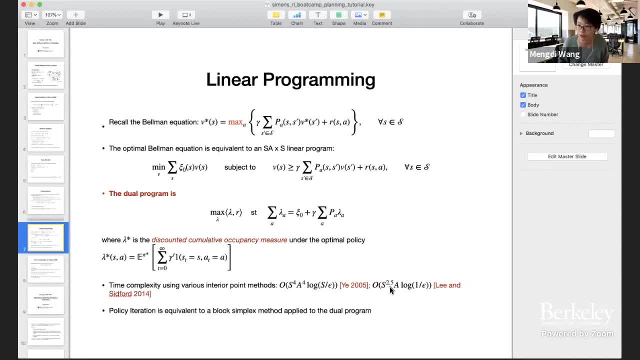 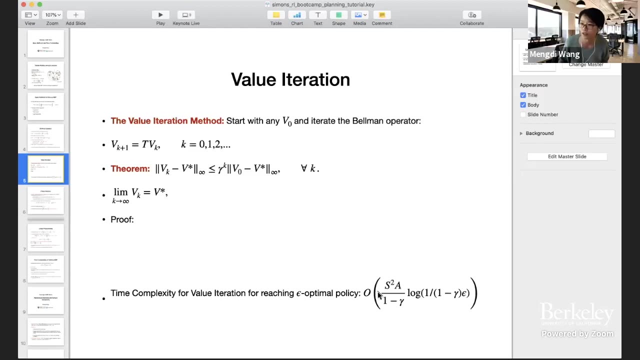 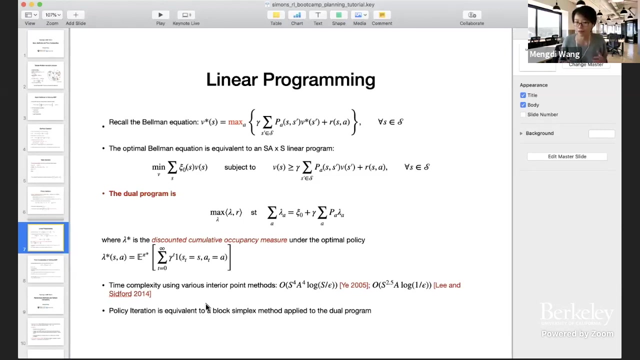 has super linear dependence on the input dimension. Okay, and comparing to the one we had this value tuition. the similar algorithm actually has linear dependence. So it might seem like LP methods might not be the perfect algorithms for solving this particular problem. So we can actually see why this is true. 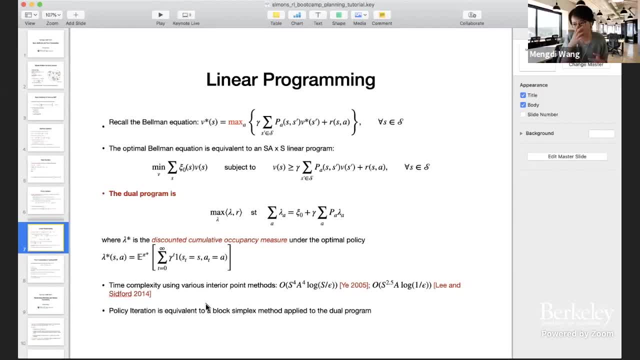 because if we're treating this problem as an LP, we're not utilizing the contraction and the monotone properties of the Bellman operator, We're only using the fact that it's a print LP. Okay, but one thing interesting is if we look at this particular dual linear programming, 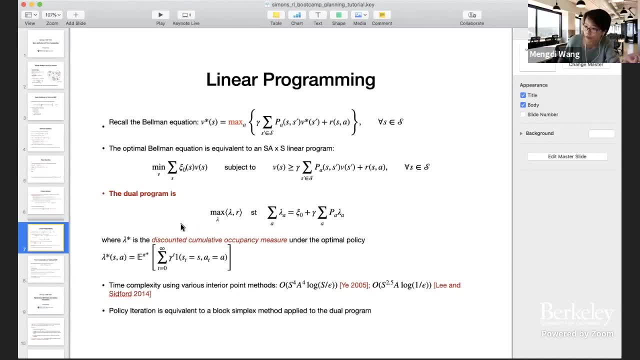 okay, we realize that we have a space of state action, opposite measures, right. And if we are familiar with LP, then this space of lambda is a big polyhedron And we have many vertices on this polyhedron And it turns out that the vertices 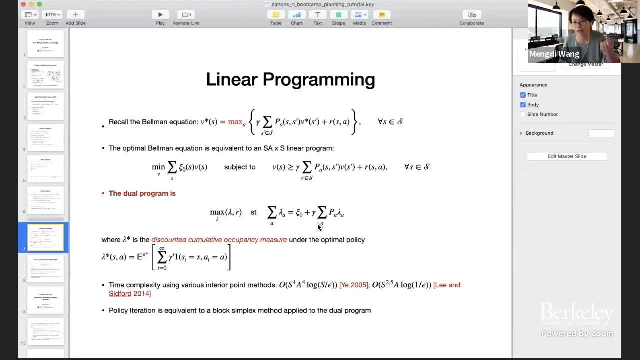 of this LP constraint corresponds to deterministic policies. Okay, and one can further show that the policy tuition, the algorithm that improves policies one by one, for that algorithm is equivalent to a variant of blocks and that it linguistic relations for r1 are approximate. 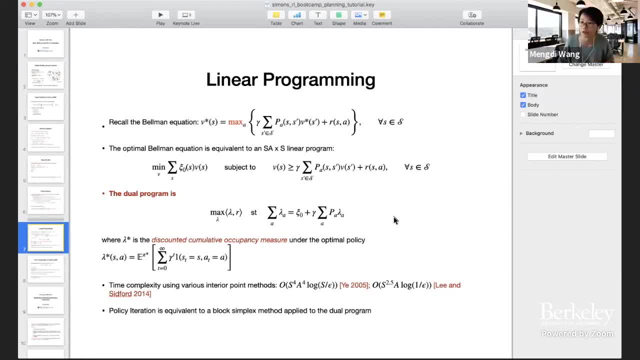 Yes, Here it's really quiterier. user learning has to me which is quite similar to the size problem, in which the idea of complex method applies to the dual problem. So there are very there are many interesting correspondences there. that's fun to analyze. 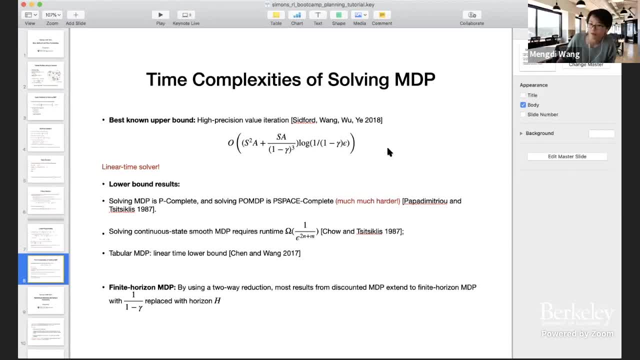 Okay, so last slide. So the best known upper, bound to my best knowledge, is this one: algorithmic hacks and randomization to help accelerate, to help accelerating it, And, as we can see, this complexity is almost linear in the input size. So we have 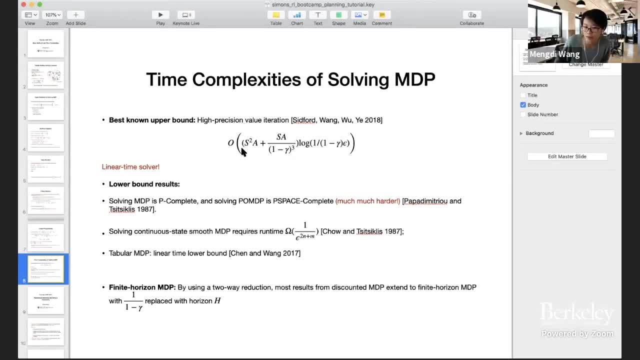 some modeling factors by this logarithm and there are some additional factors, But hopefully this is much smaller than input size. So we will say this is almost a linear time solver and it could be the best we could expect. And as for lower bounding results, So there was the seminar paper. 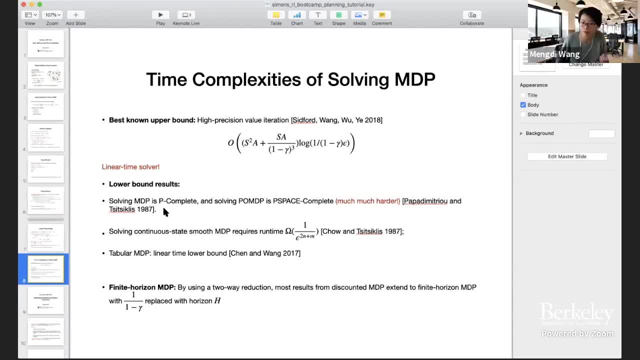 by Papadimitriou and John Tzitziklis. So they show that solving MDP is definitely a polynomial time problem and is p complete. But although MDP is simple and nice, but if we have partial observability, the problem 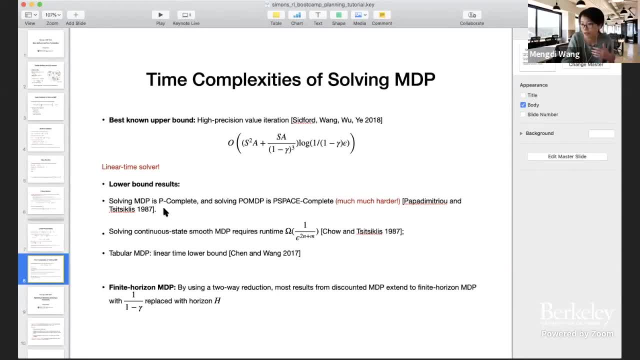 becomes really hard. So solving POMDP is p space hard. It's even harder than NP complete, So it's just much, much harder If we have partial observability. So having states that give us the Markovian property is really a blessing. 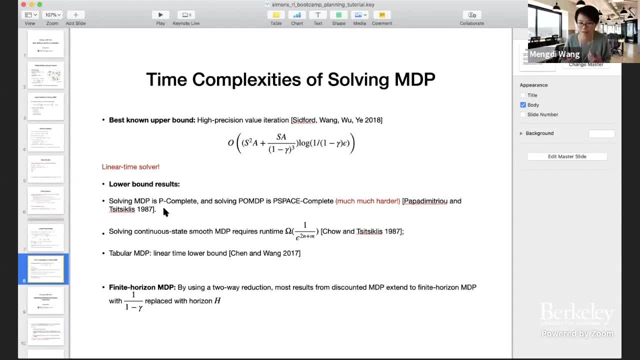 OK. And also there was this classical result that if we try to computationally solve a continuous state, continuous action, MDP- with smoothness, then the runtime is going to be like this. So basically it's going to be exponentially bad in terms of dimension of the state. 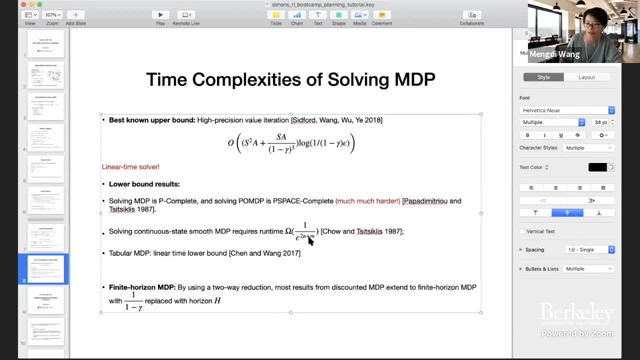 So we're going to have this constant action vector and action vector. OK, So finally, I just want to say that most of the results for discounted MDP extend pretty easily to find out how it is And so, as Chaba mentioned, so it's pretty straightforward to read- to how to construct. 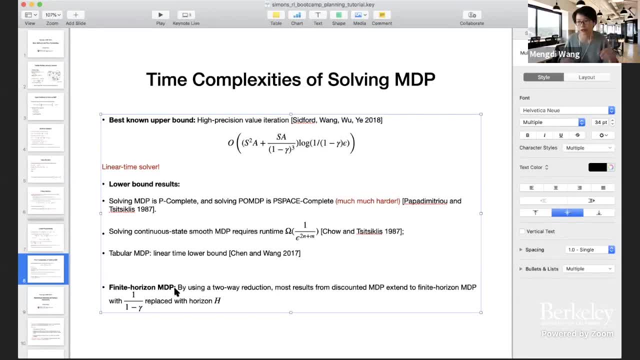 a reduction for them. Or we can always approximate a discounted MDP with a final horizon one by just choosing the horizon to be long enough to be like this. And the other way is we can always approximate a finite horizon MDT by picking a good discount factor in a discounted MDT. So those results for discounted MDT. 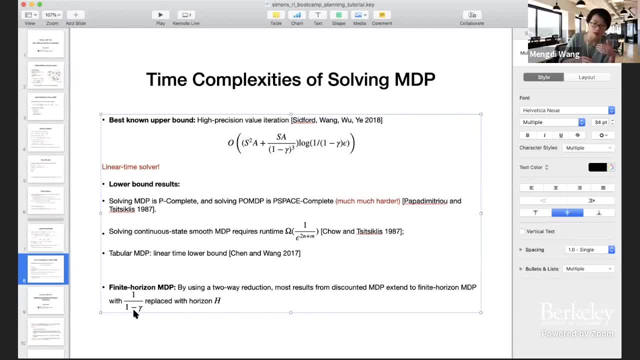 almost all hold for finite horizon, MDT- But if we talk about undiscounted infinite horizon, then the problem becomes much harder and it's not within the scope today. Okay, so I'm going to stop here and we're going to have a short break. 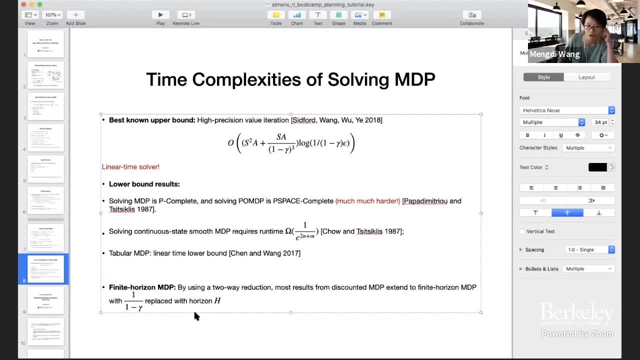 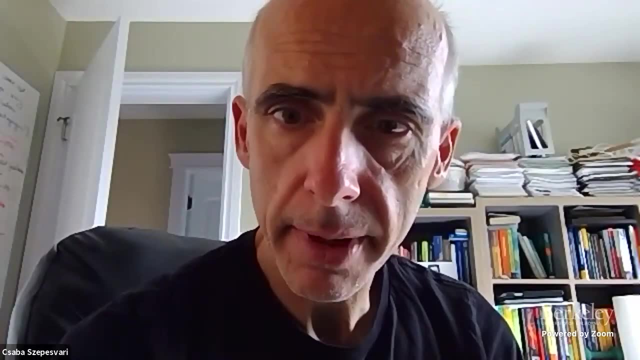 and then we'll continue in probably 20-30 minutes, Right? so there is this Getter Town link. It was posted in the chat somewhere. I think you should just head there and then we can continue having some conversation there. Okay, I'll be there. 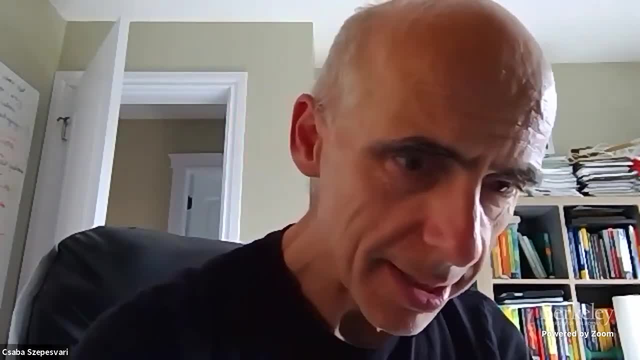 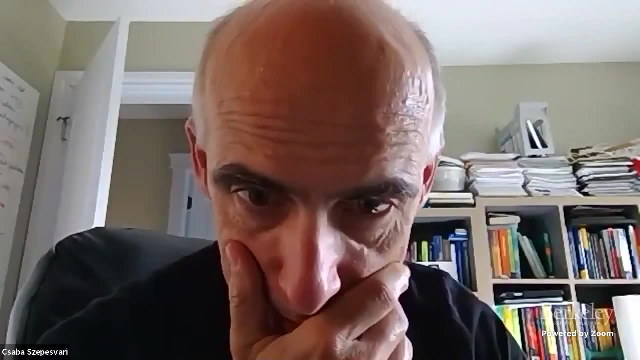 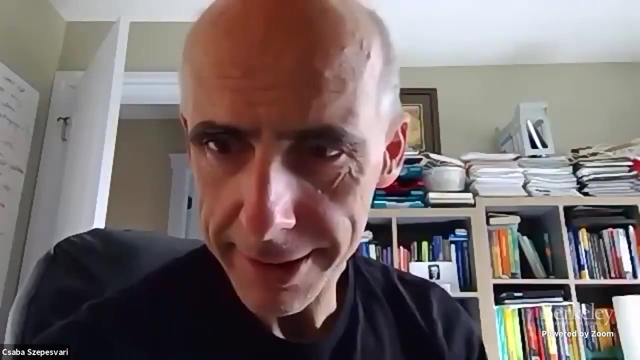 See you soon And then we come back in 20 minutes. Okay, so there is the link again. If you haven't used Getter Town, you just click on this and then you are a little avatar and then you can go near people and then if you're near to someone, then you can talk to them.